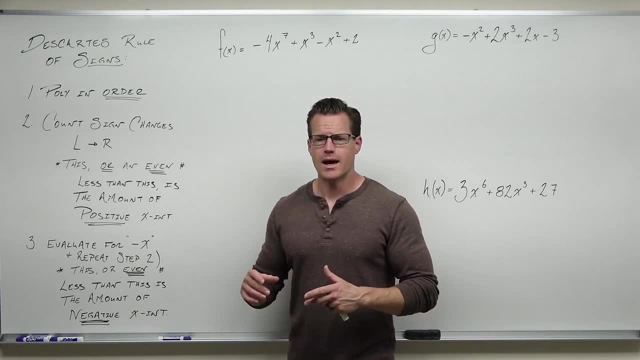 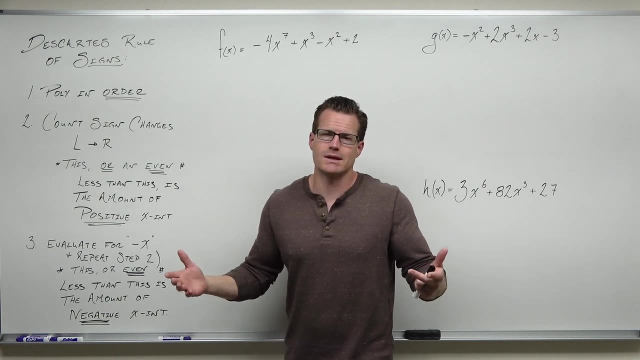 concept in there because I'm going to be referencing it in the next video And it's important for you to understand because I want to save you time. I don't want you to waste a lot of time checking things that you don't need to because they don't exist. It'll give you a better understanding of 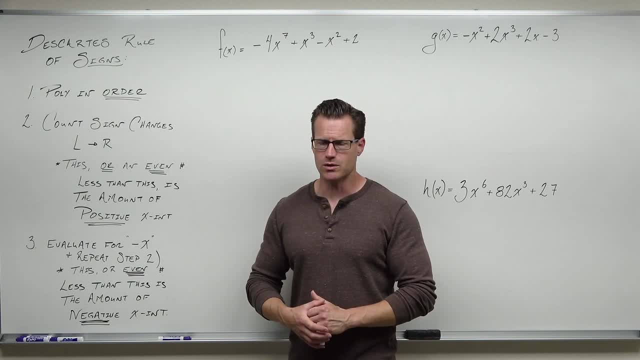 what is going to happen when you start factoring these polynomials. So we're going to get right into the Descartes' rule of science. I'm not going to prove it for you. I will tell you the idea behind it, though. 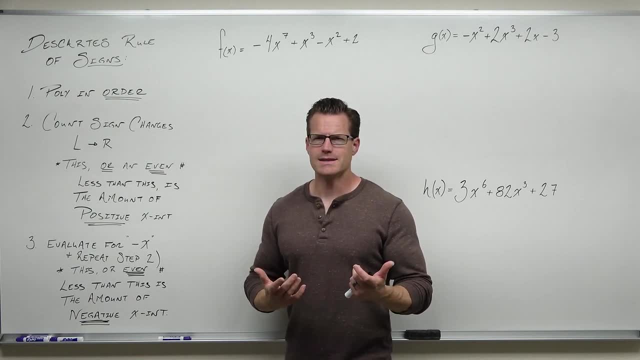 So, as we go through it, I'm going to explain to you why is it that you can have three positive x-intercepts, or one but not two and not zero, or two or zero but not one or three, why it decreases by an even number. And so here's what you're going to learn in this video. You're going 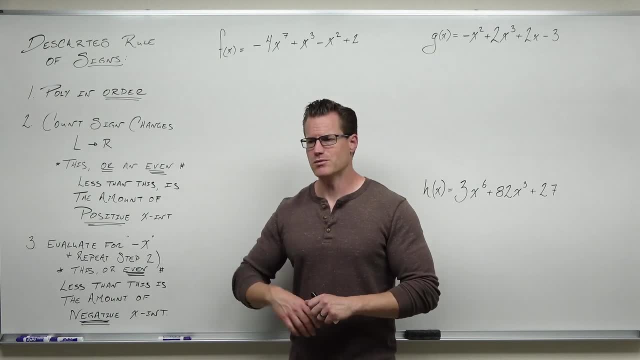 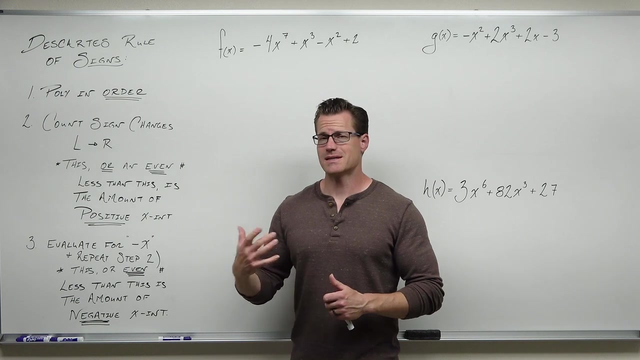 to learn that if you have a polynomial in order and you just count the number of sign changes from left to right, it will tell you the number of positive x-intercepts you have. Real, It's going to tell you either have like three or one or that's it, or maybe six or four. 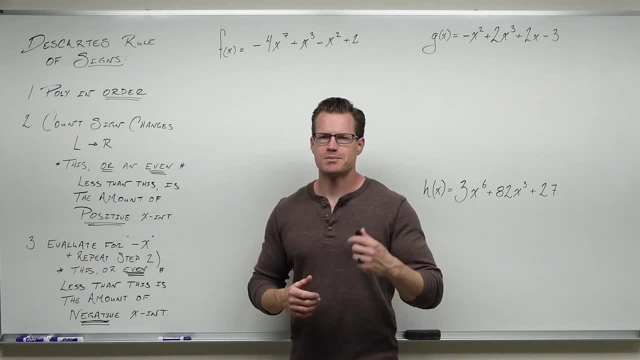 or two or zero, You know what. That might not be that powerful. It's powerful when you start combining it with rational zeros theorem. When you start finding zeros, it'll tell you how many are left. or maybe it'll tell you there's no positives or no negatives, And that's very 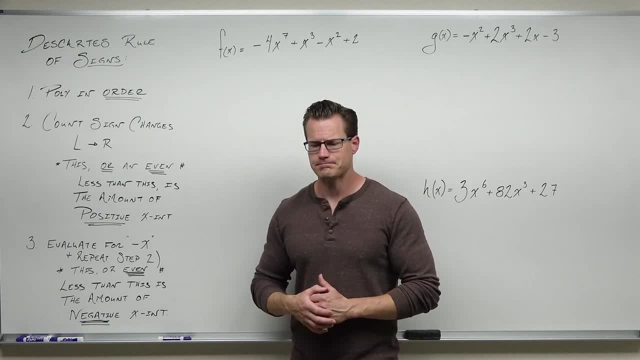 important because we can eliminate checking values that would not be x-intercepts anyway. And so that's what we do. We change the signs of our odd exponents. Why? Because you're going to evaluate for negative x. All that does is change the sign of your odd exponent terms and do the same thing, Only this. 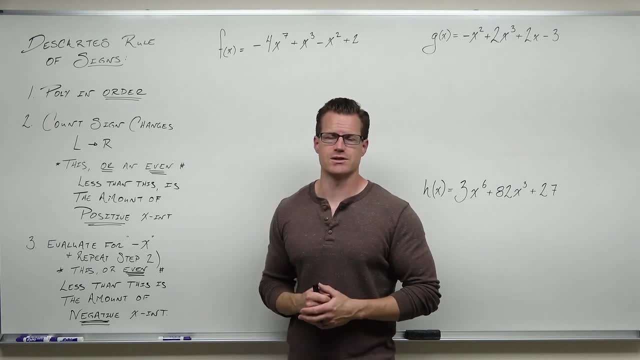 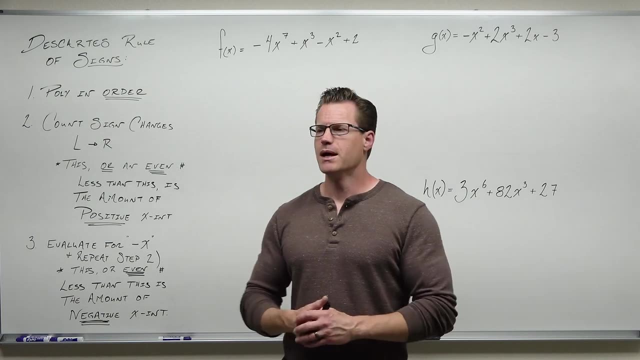 time. it's going to tell you the possible number of negative x-intercepts. That's what the Descartes rule of signs basically does. So we're going to get right into it. So what we're going to do, we're going to put your polynomial in order every time. Now, if we're going to count number of sign, 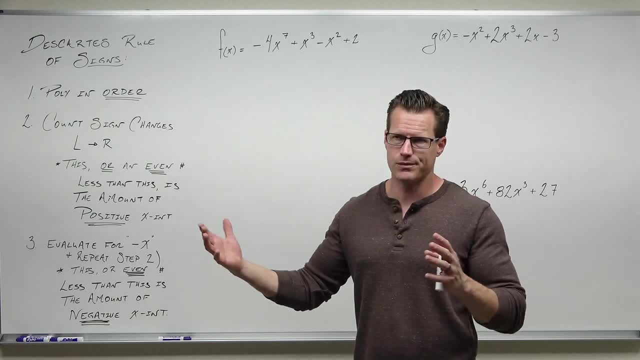 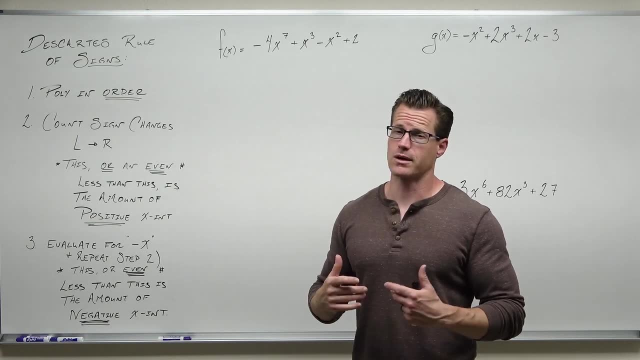 changes. that's very important. You want to make sure they're in order. We do that anyway for basically everything we do, But it's super important here, So make sure your polynomial is in order before you start any of this stuff. Then we're going to count the number of sign changes from left to right. So let's look. 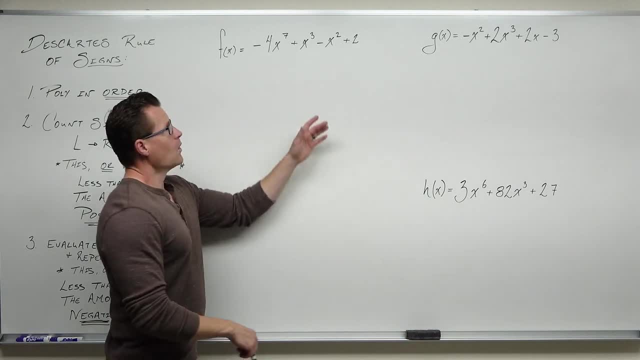 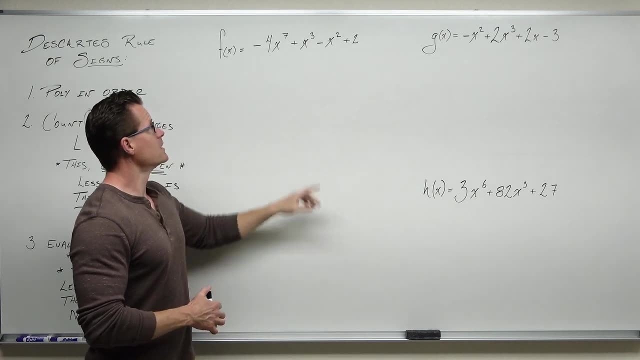 at our first example from. well, first we check order. Order means your exponents are decreasing until you have a constant. If you have a constant, it should be a blast. So seven, three, two, zero, That's fantastic. That's what we want. Then we count. the number of sign changes from left to 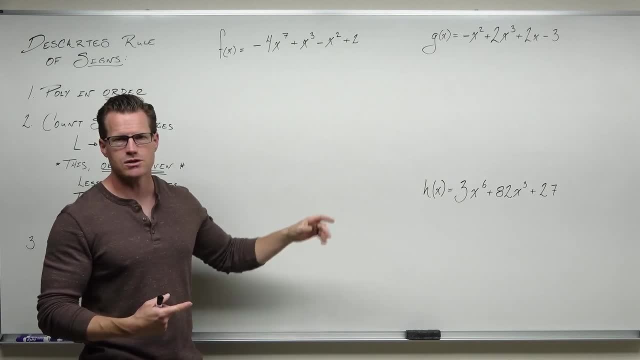 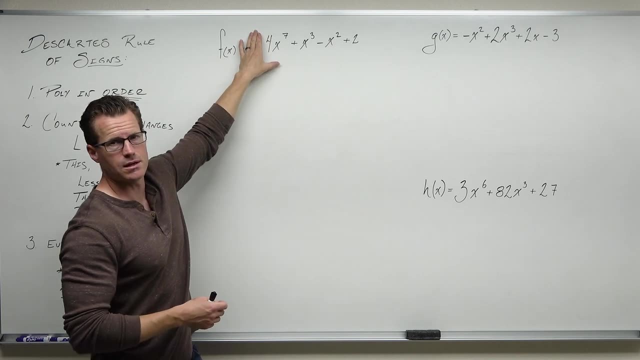 right, So we go okay. well, what is it? What does that mean? You look at your signs, So I I gave you, starting with a negative, so that you can see that that is a signed term. If that negative wasn't there, we would consider that to be a positive And we might even write a little plus. 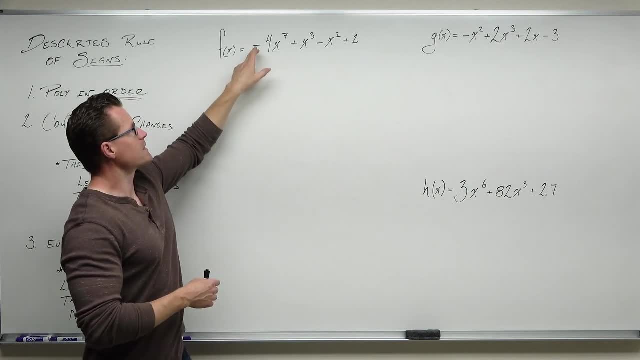 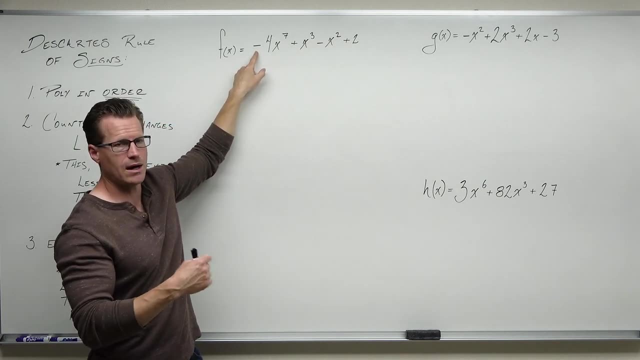 in front so that you can see what's going on. So this is a negative, That is a plus, a minus and a plus. So, as we're counting from left to right, you say, okay, that's a negative, We have not started really counting changes yet, because you start somewhere, So we say that's a 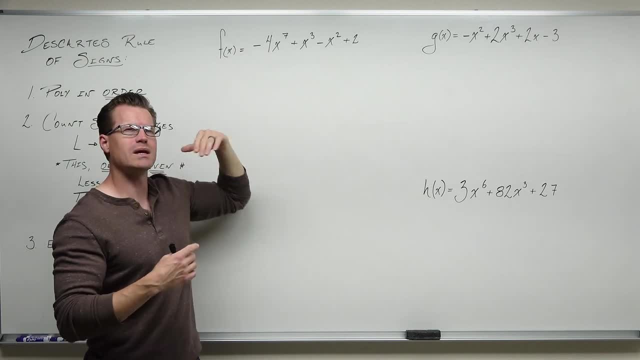 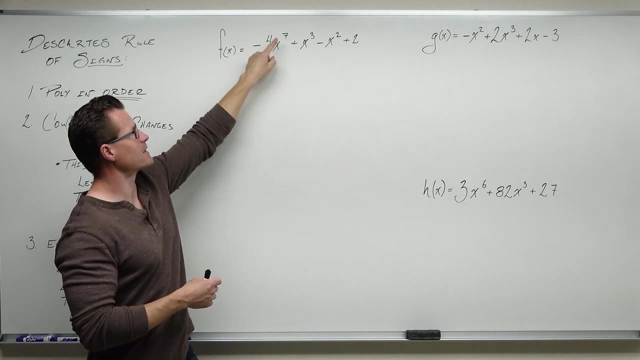 negative. What's the next sign? Is it the same? Or we can say: is it, is it uh? could it be written as a negative, or is it a positive or a plus? So we say that's a negative, That's a plus. 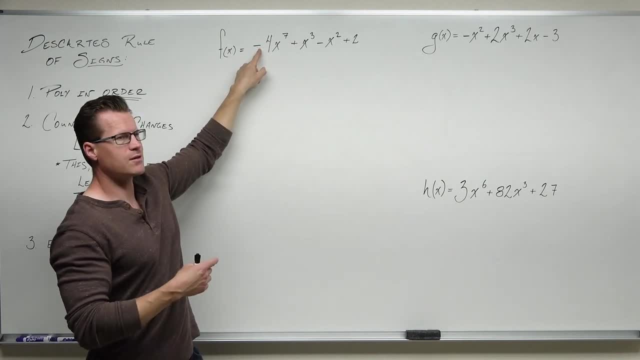 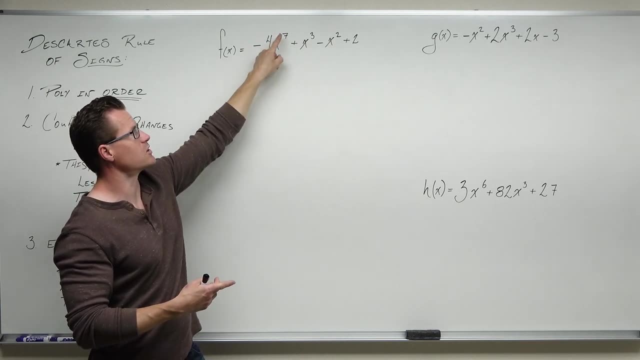 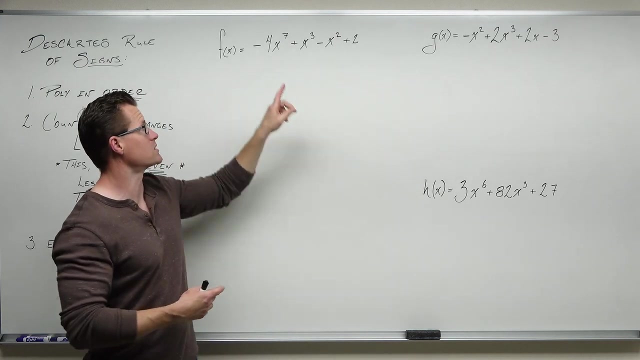 This counts as a sign change. You go: okay, think of this as negative or minus, Think of this as positive or plus. this would be negative to positive. That is a sign change. One. positive to negative, That's two. negative to positive, That's three. There are three sign changes here. 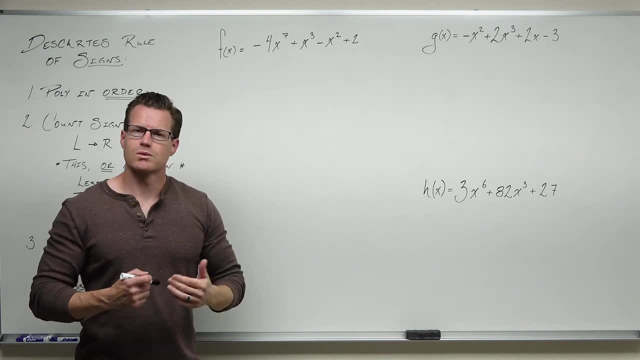 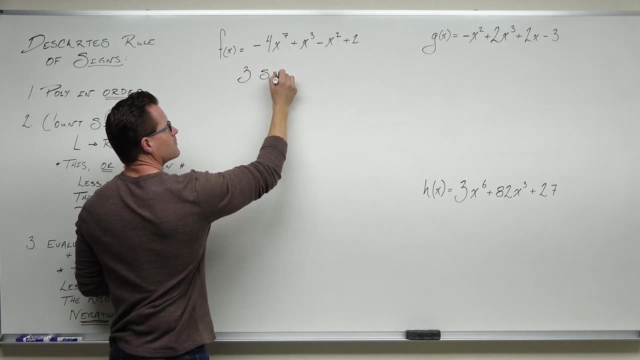 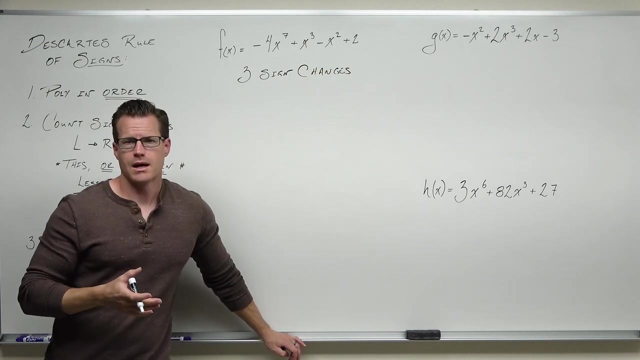 One, two and three. So here's what we're going to say. We go all right, there are three sign changes. What that means is that in this polynomial, if you were to graph it or you were to solve it, you are going to have either three. That's what this says right here. It's very wordy. 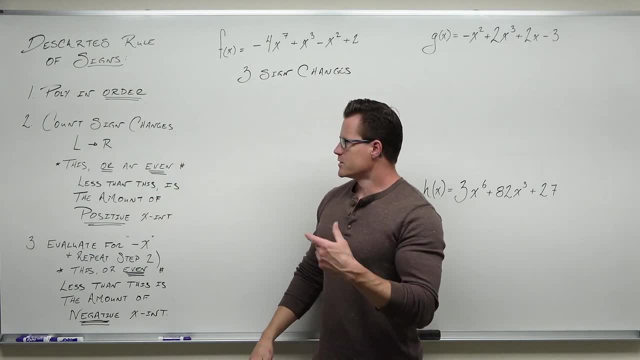 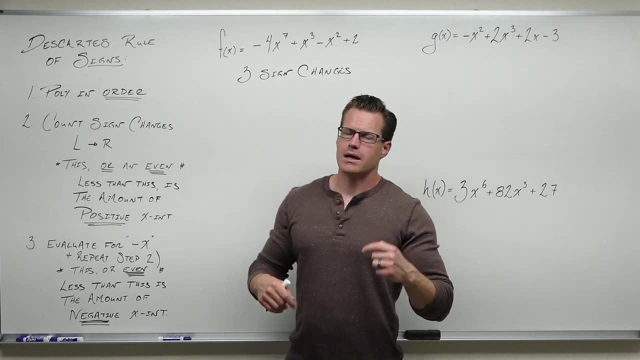 And when you read the first time you go: that's making sense at all. Um, you are going to have this number of sign changes or an even number less And that amount. you know what does that mean? Even numbers are two or four or six, So all you. 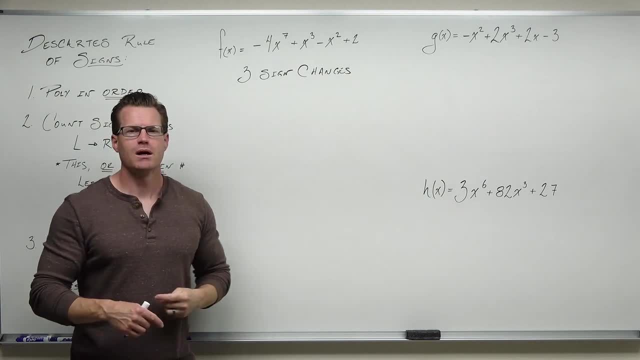 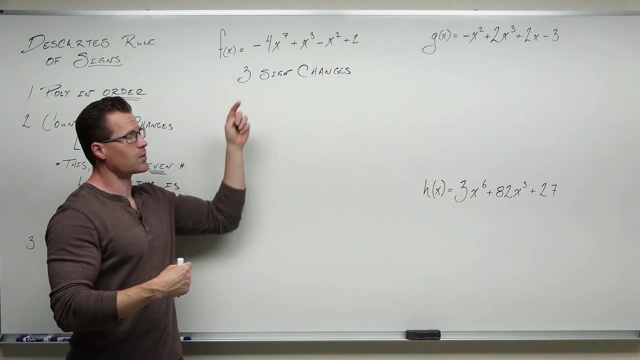 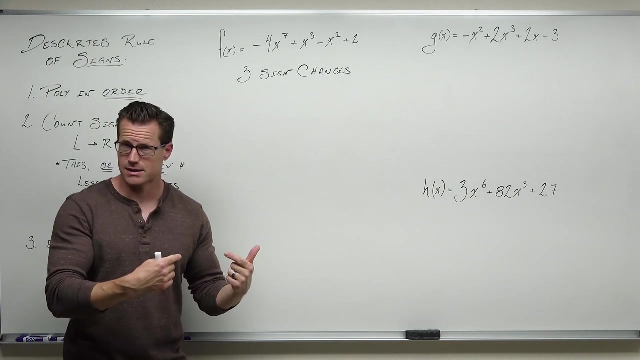 really do is you count the number of sign changes. Hey, there's three. You could potentially have three sign changes, or keep subtracting two from this number until you hit either one or zero and then stop And you will have a list of the number of positive X intercepts you could get. So we 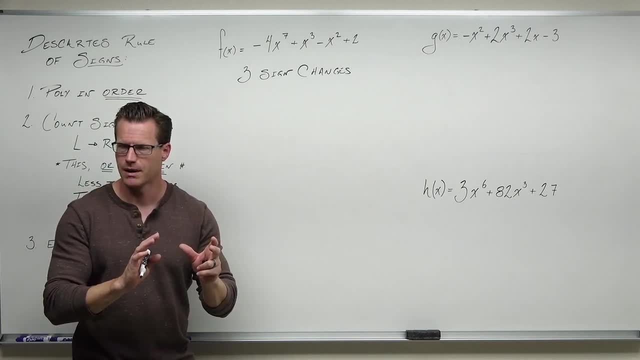 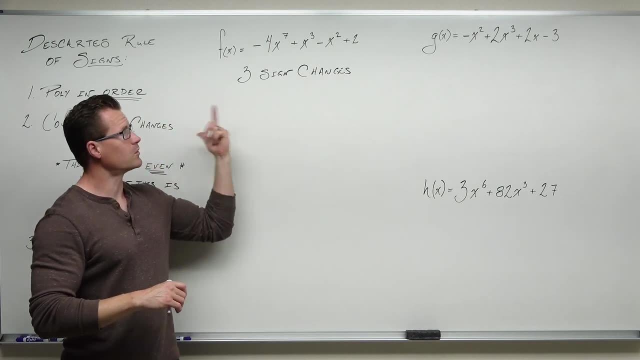 said: all right, I know that this can be the confusing the first time you hear it, Um, so I'm going to kind of repeat myself several times in slightly different ways, so that it clicks in your head. put it in order. We got to count the sign changes. That's the most important thing, uh. 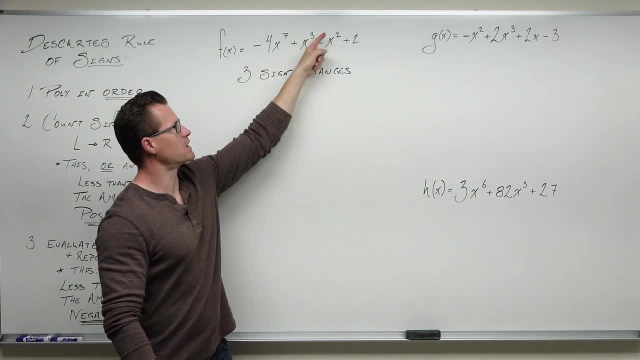 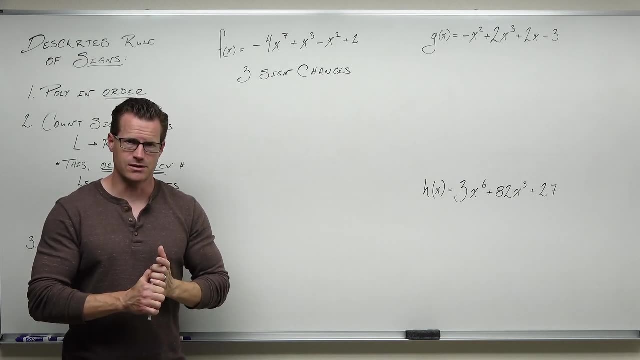 besides interpretation. So okay, Uh, one sign change, two sign changes, three sign changes. You write that number down. That number that we write down represents the number of positive X intercepts, or any even number less than that represents the number of positive X intercepts. 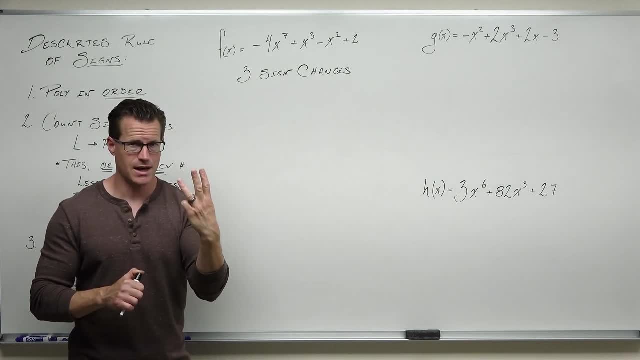 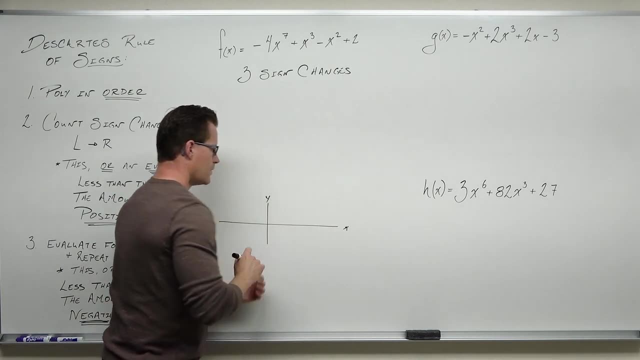 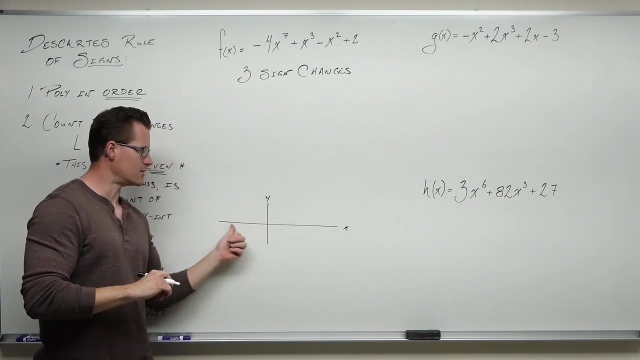 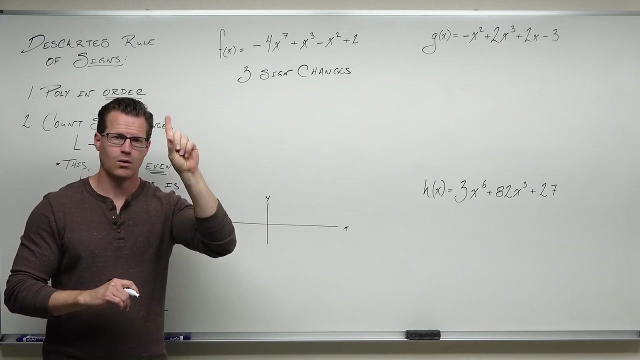 So there could be three positive X intercepts. If you remember, this is the X axis and this is the Y axis. This would be considered the positive X axis and the negative portion of the X axis. What this says is there will be three or one positive. 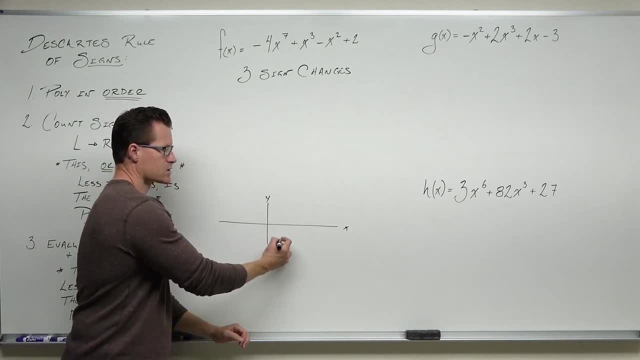 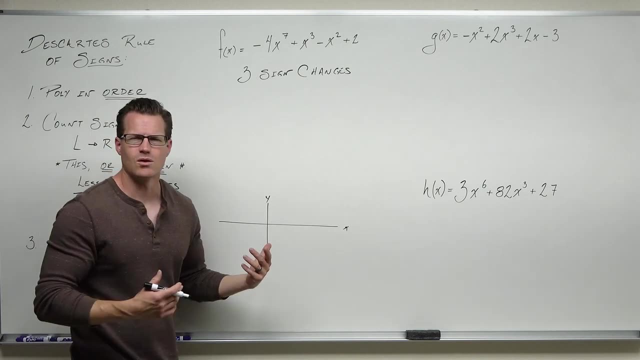 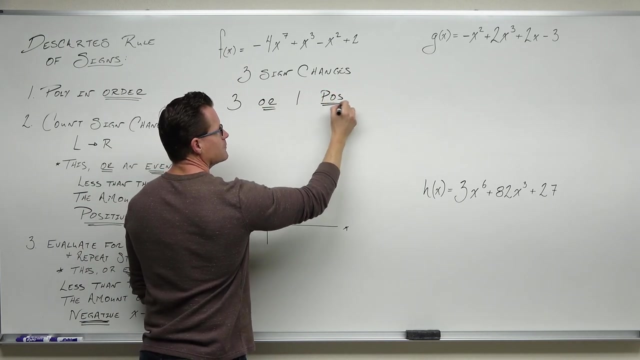 X intercept. It's either going to cross or bounce one time or three times, not two, not zero. one, three or one. now how to? where do I get the one from? So there will be three or one positive X intercepts. Where do I get the one from? That's where this comes in, right here that. 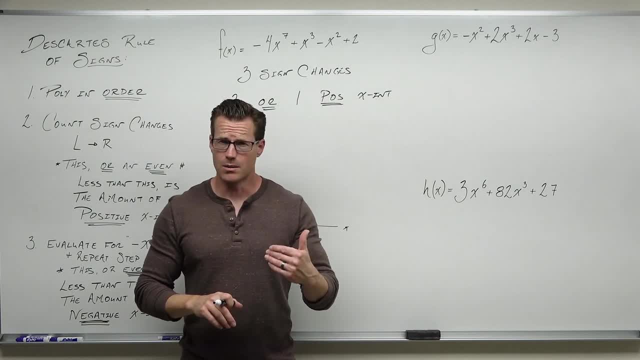 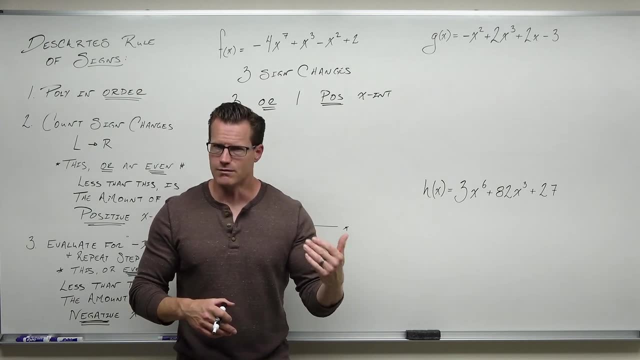 or an even number less than this. So you write down the number of sign changes like three. you go, okay, start subtracting two from that. two is an even number And every multiple of two is an even number. So you go, okay, if I have three sign changes, they're. 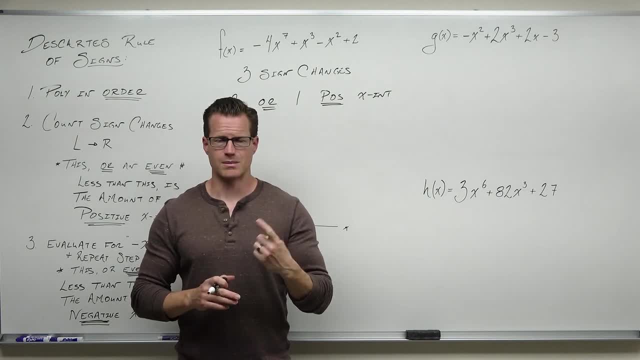 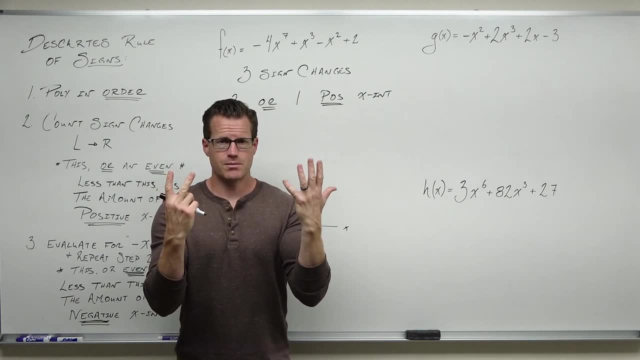 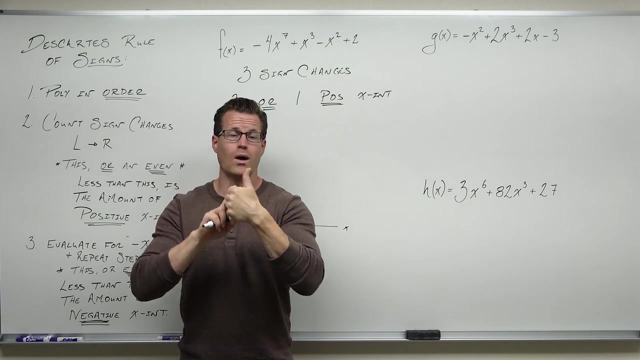 three, or subtract two, one positive x-intercept. Let's say you started with seven. If you had seven, sign changes you go. okay, there are either seven positive x-intercepts or five. take away two or three. take away two or one. That's the potential number of positive x-intercepts. 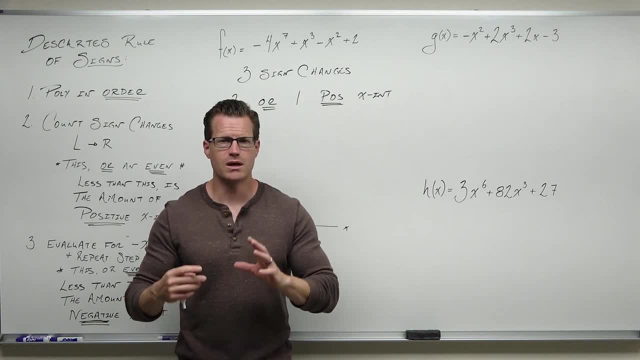 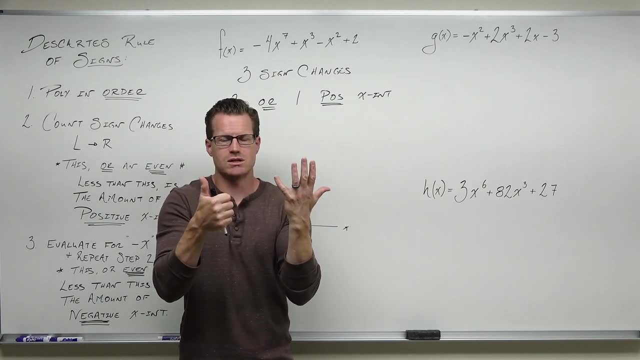 that we would have. Now it's not going to be all of those, It's going to be one of those: either seven or five, or three or one. What if you had like six, like six, sign changes? Well, you'd have either six positive x-intercepts or take away two, four, or take away two, two or 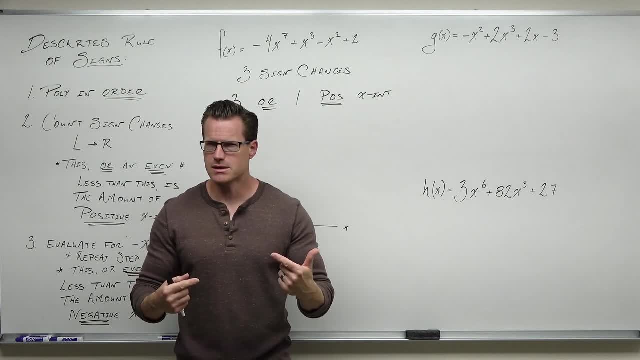 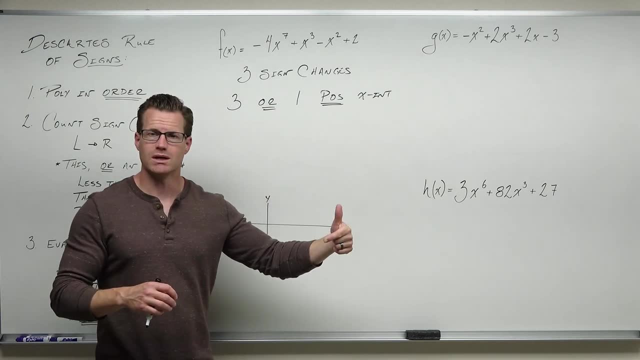 take away two, zero, So you come up with sort of a list of how many positive x-intercepts you could get. So count the number of sign changes. three: write that number down and just subtract two until you get down to one or zero, depending on whether you have an odd number. 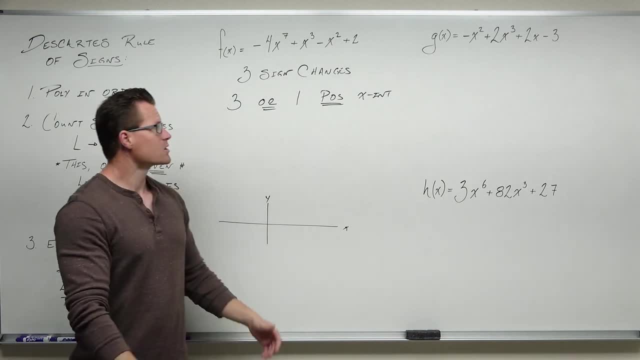 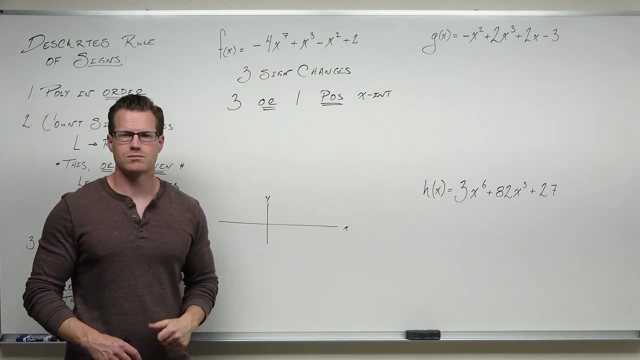 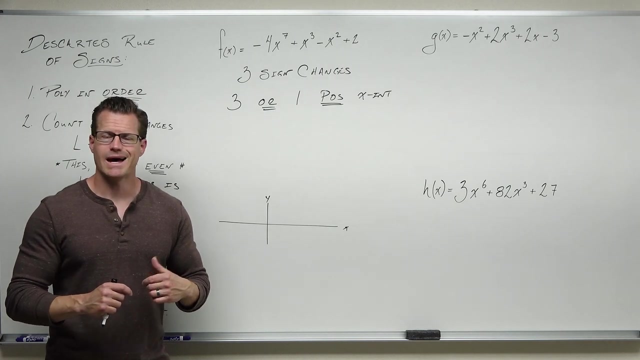 um sign changes or even number sign changes. So what this says is that we can either intersect the x-axis on the positive portion of it one time or three times. three times or one time. That's it Now. here's why that's important. We know for sure that we're going to have at least 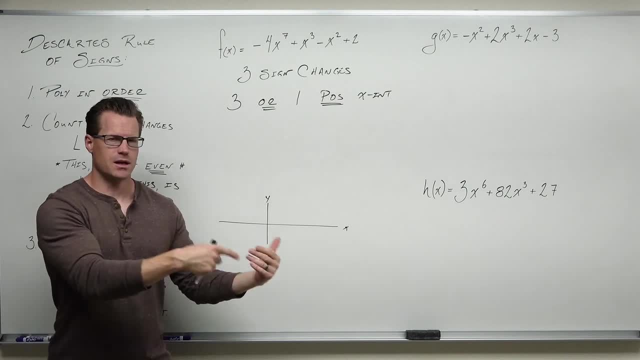 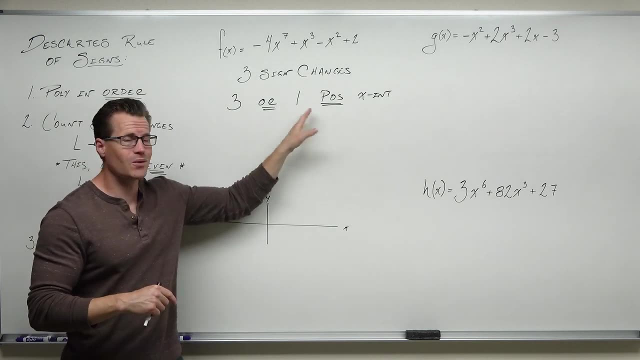 one positive x-intercept. So when we go check numbers in the next video, I'm like: ah, what number is going to work? We would want to include positive values, because you are going to have one. This is why we can't get to zero. This is why we don't put zero up here, because, um, one minus two. 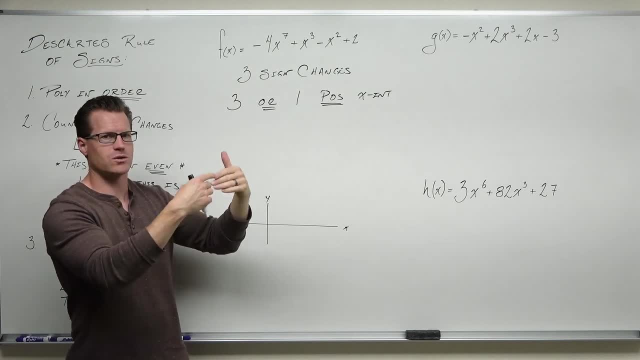 is it surpasses zero. You can't just subtract one and go: oh, it's three or two, or one or zero. You're going to have either three or one, right, That's? that's your guarantee. You're going to. 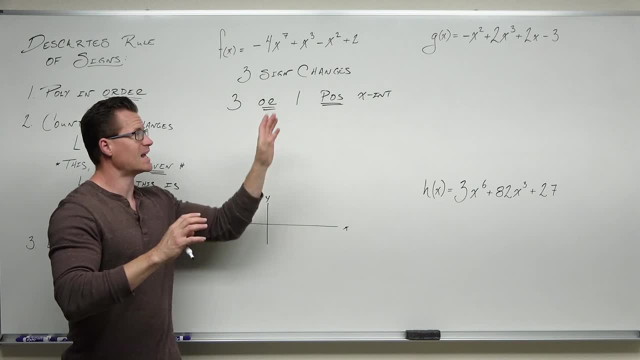 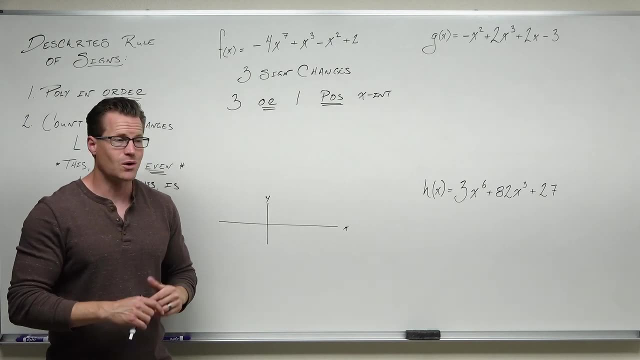 have either three or one positive x-intercepts. You're going to have at least one of them, possibly three of them, no more than three, no less than one, And you're not going to have two. So it's one or the other. Um, so you would want to include those because you know. 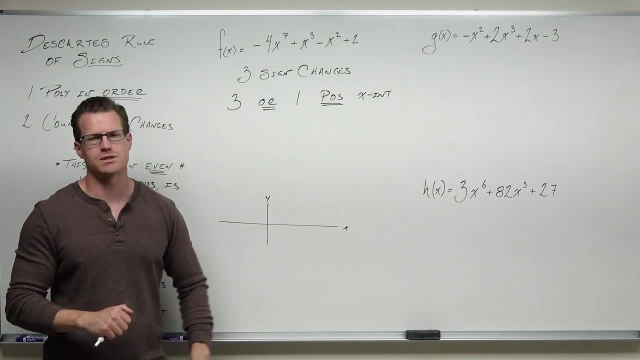 you're going to hit somewhere over here at least one time, possibly three times, but that's the only options for you. Now, a common question is: why in the world do you subtract two? Why, Why two or four? Um, what that has to do with is irreducible. 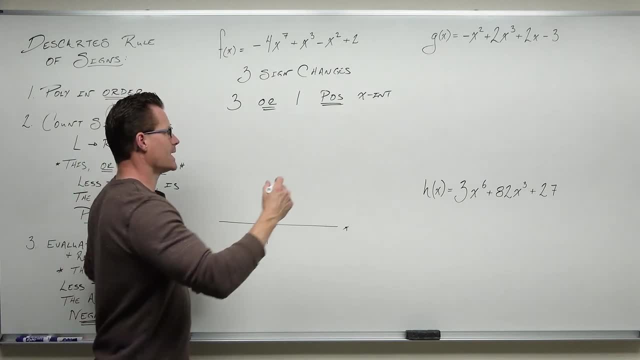 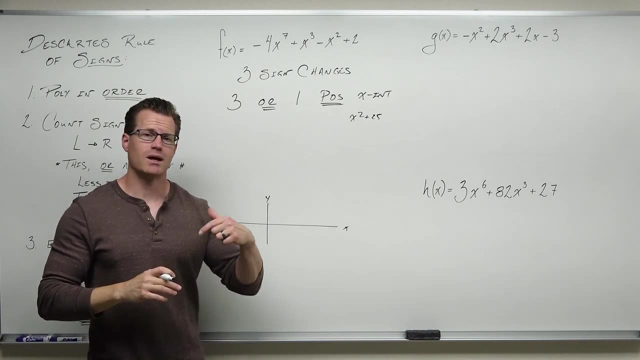 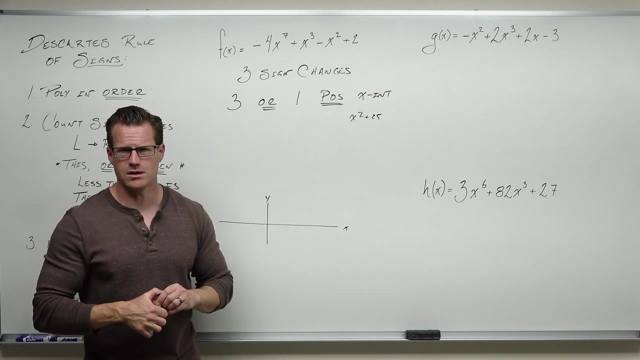 quadratics, So irreducible quadratics like x squared plus 25, you cannot factor that. That does not give you any additional x-intercepts, but what it does is subtracts from your, your degree. So if you remember this, you do need to know this- Your degree represents the total number of x-intercepts you could. 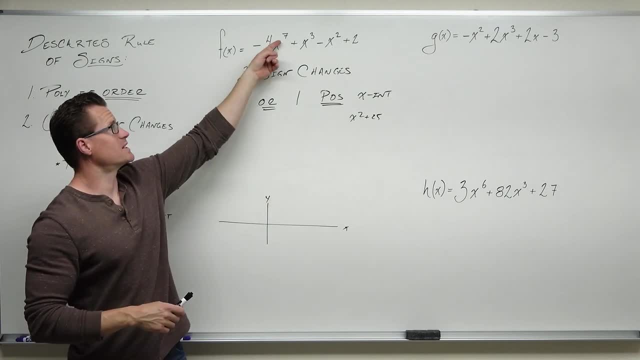 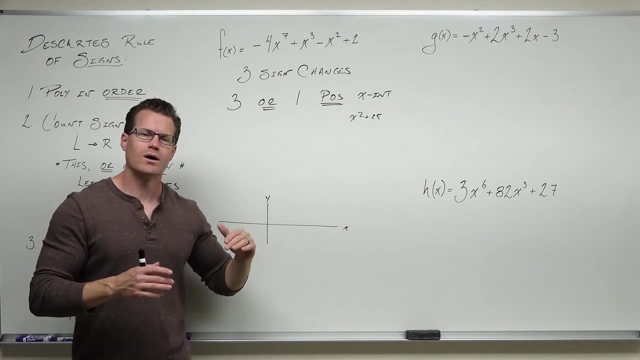 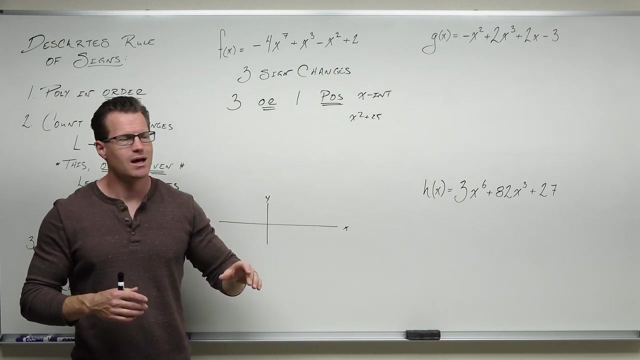 possibly have. So this says you could potentially have seven x-intercepts. Are you going to have that many? Not necessarily. Why? Well, because irreducible quadratics give you complex zeros but no x-intercepts. They do things like they create these um, these local maxima and minima. 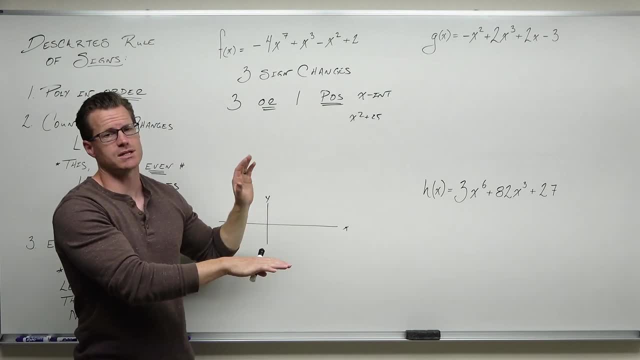 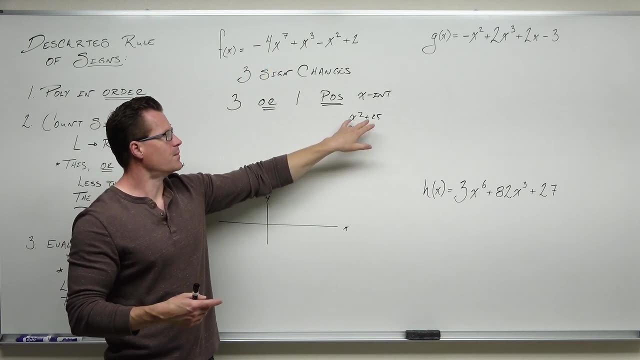 somewhere above the x-intercepts. So you're going to have seven x-intercepts, So you're going to have the x-axis where it doesn't cause an intersection, or below the x-axis, And so what that does is this counts for if this is a factor, I don't even know, but what this would do is this would take. 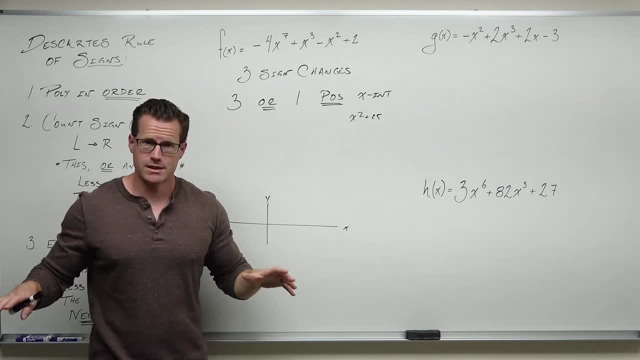 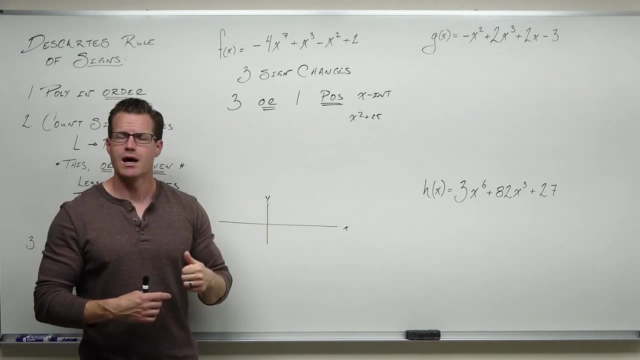 away two from your degree if you start factoring it, but give you no x-intercepts. And for that reason- that's, that's basically the reason why you subtract two from this number of sign changes. because if you're going to miss one x-intercept, you're going to miss two at a time. You're never. 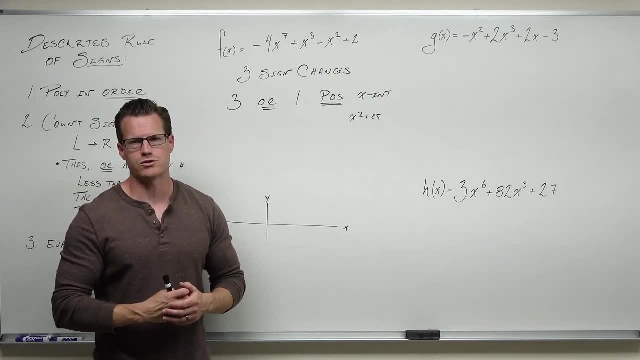 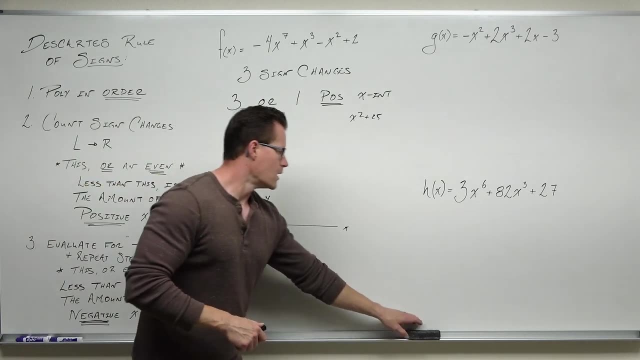 going to just miss one x-intercept at a time because of those irreducible quadratics. That's why we subtract two from the number of sign changes. I hope that makes sense. I might mention that one more time as we go through. So, all right, um run down one more time, put it in order. We. 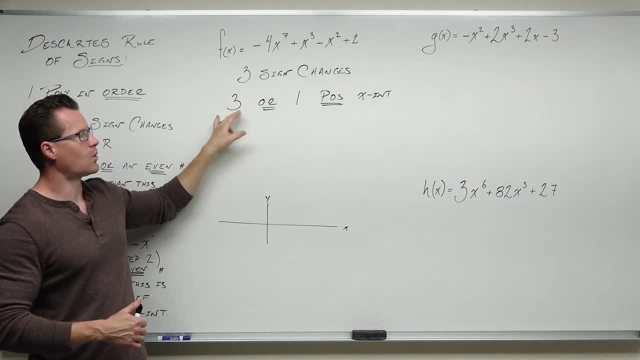 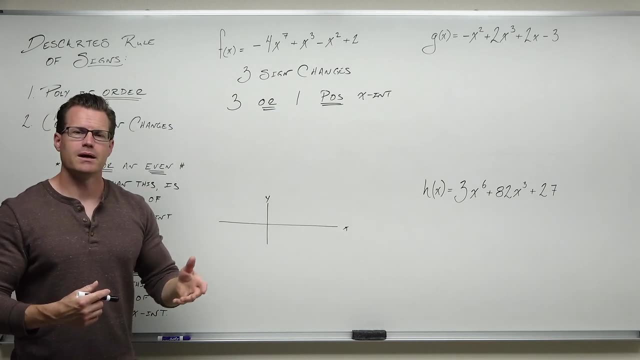 got to count the sign changes. Cool, You're going to have that many or two less than that as you and you write the whole list. So three or one positive x-intercepts. Then what we do is what we we evaluate for negative x, kind of like evaluating for an even or odd function. We say 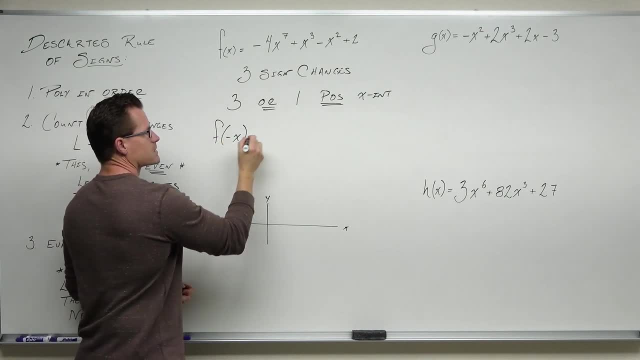 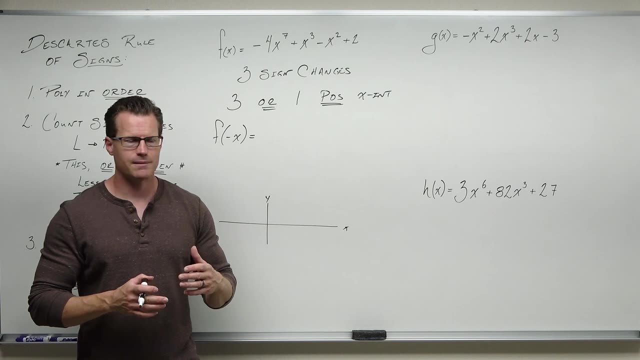 what about f of negative x? Some people get really confused on this and go: oh, I'm really bad at evaluating. I'm going to give you a trick for this. Don't even worry about it, Don't even evaluate, Don't even plug in negative. 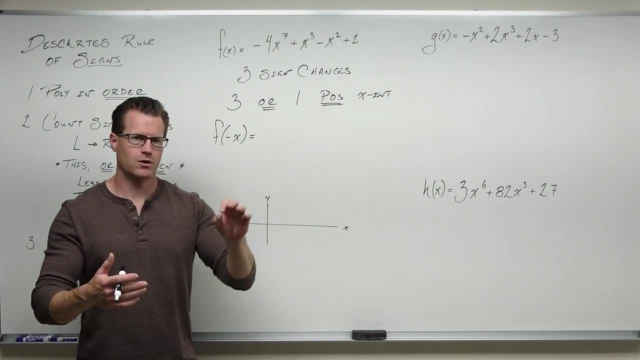 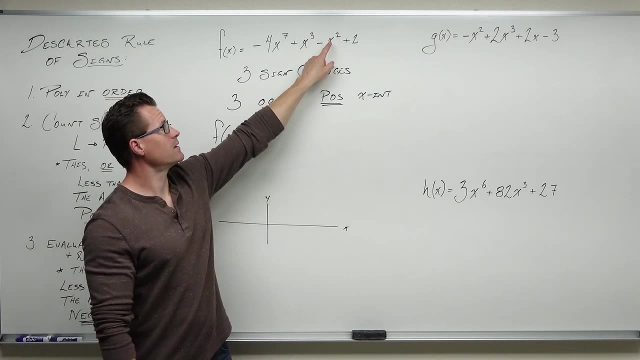 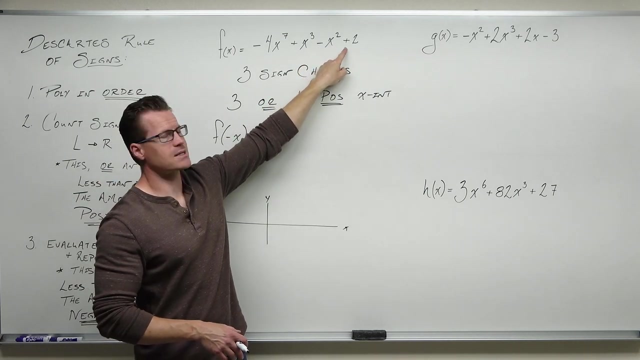 x. Just change the signs of your odd powered terms. And here's why If you evaluate negative x into an even negative, anything squared gives you a positive. It's not going to change that sign. Constants never change, sign You can't. you can't evaluate that. 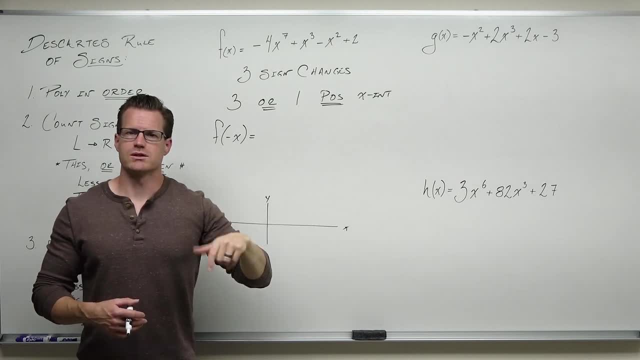 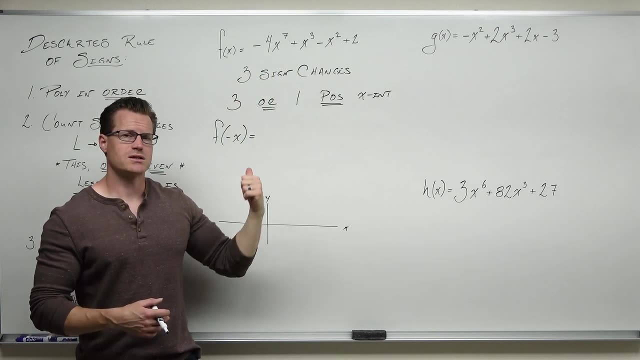 But odds, when you plug in a negative there it will change the sign. So if I plug in negative x to x cubed, it'll give me negative x cubed And I'll change that sign. If I plug in negative x to 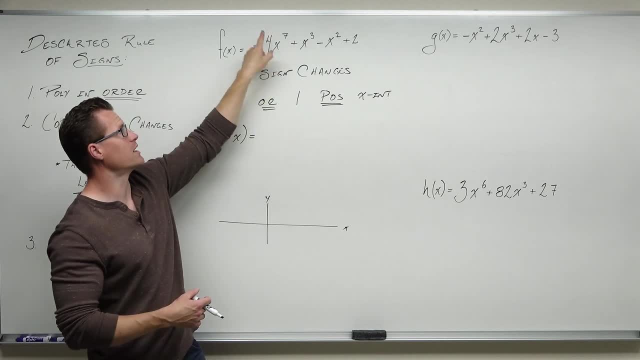 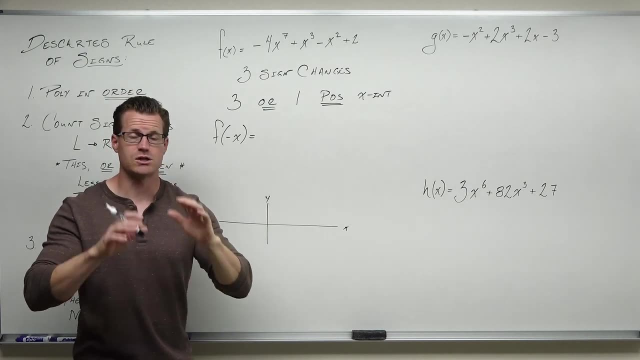 x to the seventh power, They'll give me negative x to the seventh power and we'll change that sign. So how to evaluate this easily? Just change your odd- not your even, not your- constants- your odd powered terms. change the sign in front of them. So if I'm going to evaluate f of negative x, 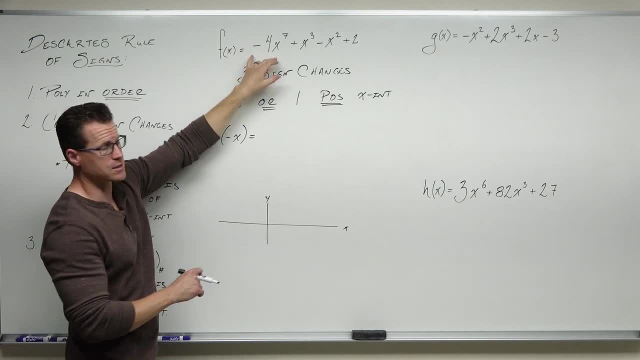 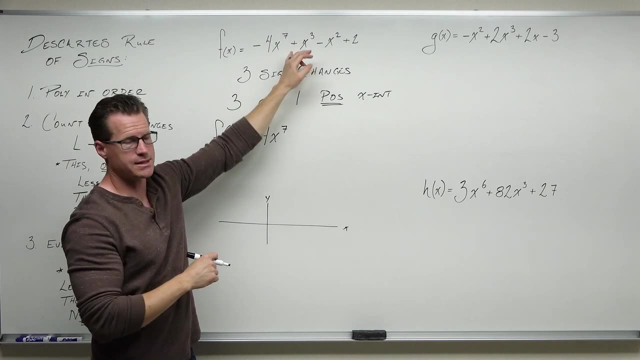 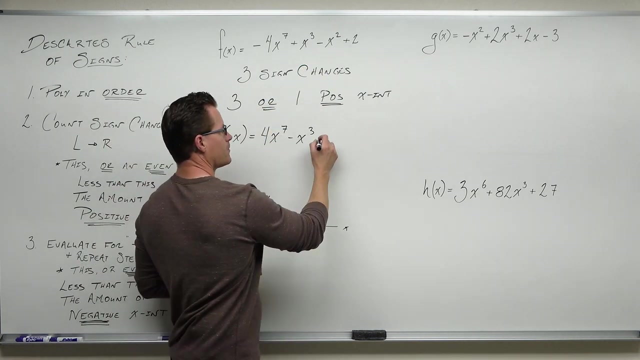 I'm going to. this is an odd power term. I'm going to change changes to positive x to the 7, 4x to the 7.. This is an odd power term. I'm going to change it to minus x, cubed. I won't change this even power term, because even powers don't. 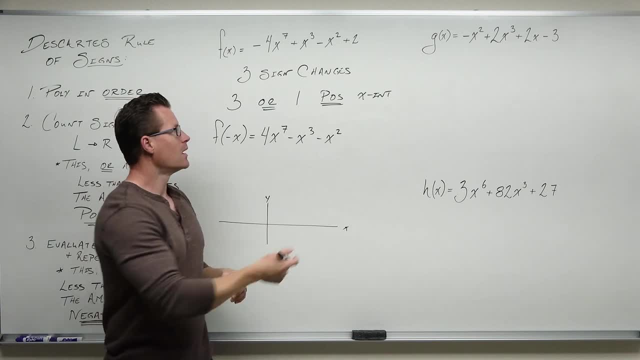 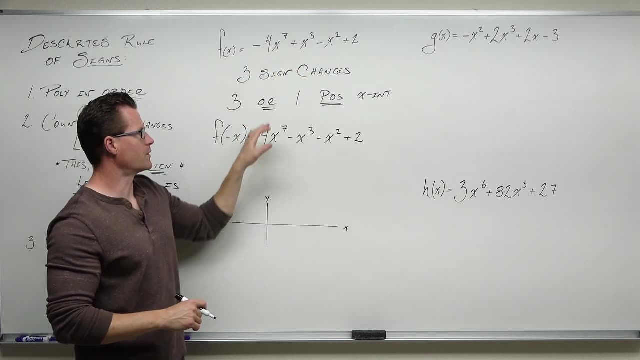 change signs. when you plug in a positive or negative, They're even. I'm not going to change my constant because there's nothing to evaluate there- And so I just look at it, change my odd power terms, the signs of those odd power terms, and then I do the same thing, But what? 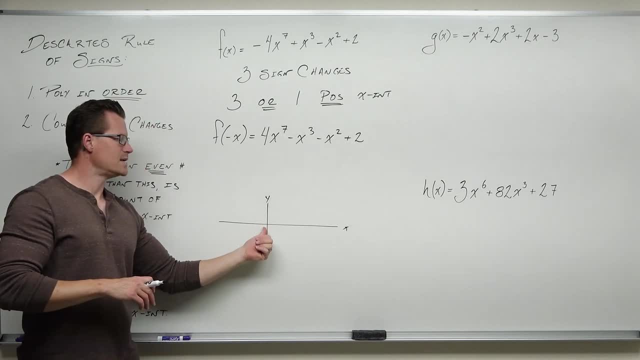 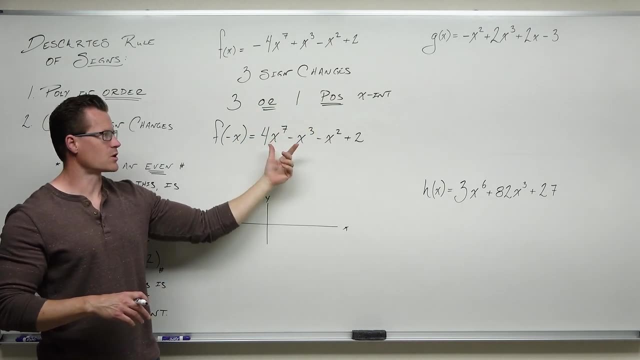 we're going to get here is we're going to get the number of potential negative x intercepts. So positive, cool, gives you a number of positive. That's pretty convenient. Change the sign of your odd power terms- That's evaluating for negative x- And then do the same thing: The number of sign. 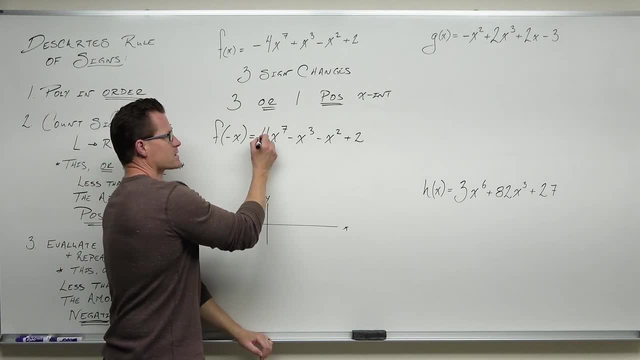 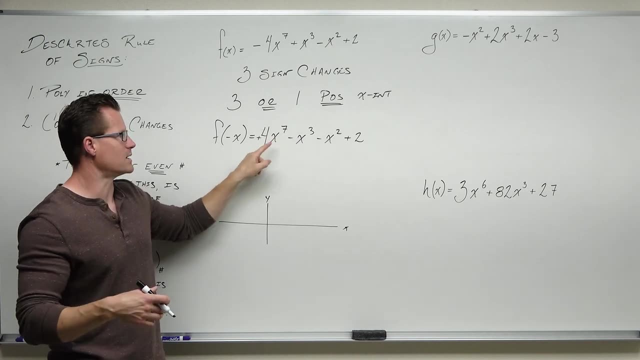 changes here are- and this is what I was saying earlier- maybe write a little plus for the positive, That way you can see the sign change. That's a positive, Or we can think plus, That's a minus. What we can think. 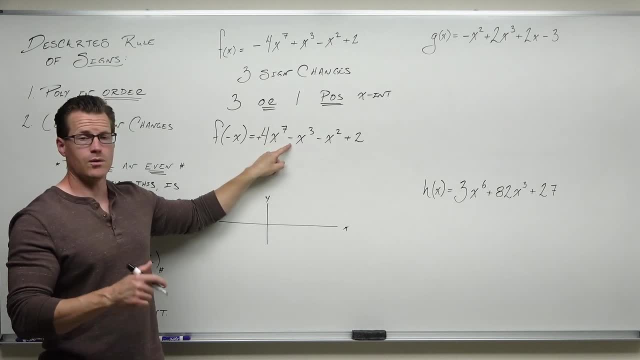 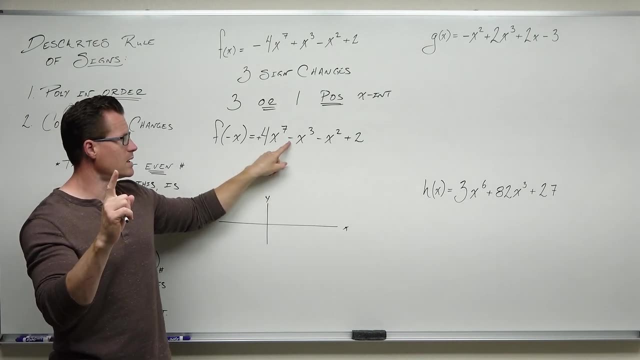 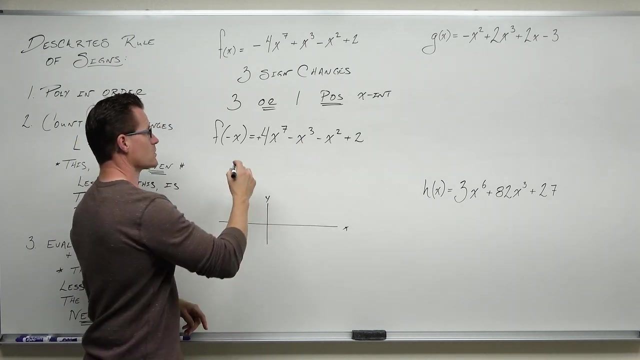 negative. The sign change. positive to negative, Oh, that's one. Negative to negative, That does not change. So positive to negative, that's one. Negative to negative, that did not change. Do not count that. Negative to positive, that's two. There are two sign changes here. 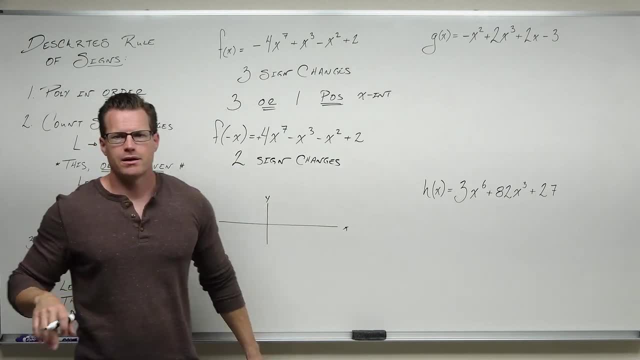 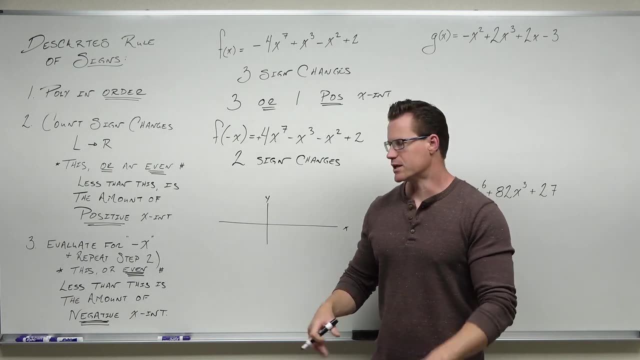 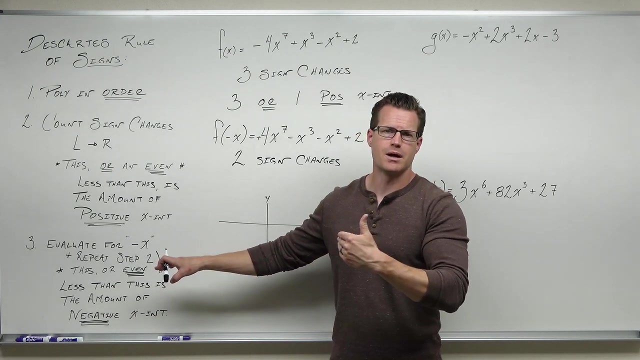 What does that mean? Because we evaluated for this negative x and we repeated this, We counted from left to right. We said, all right, there are two sign changes. Then this number represents the number of negative x intercepts, or an, even a number less. 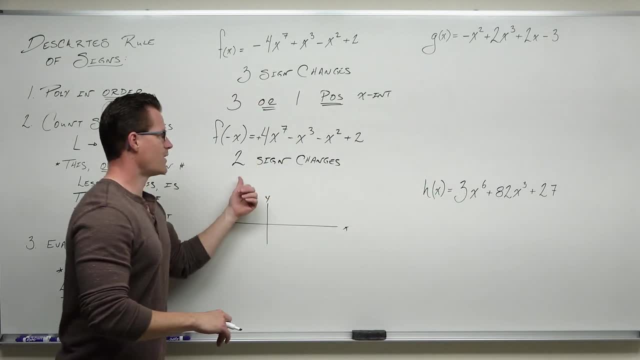 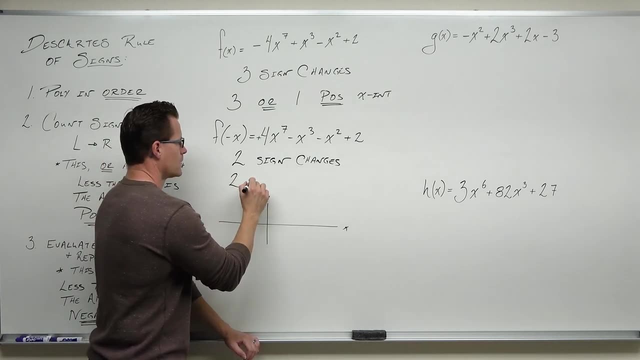 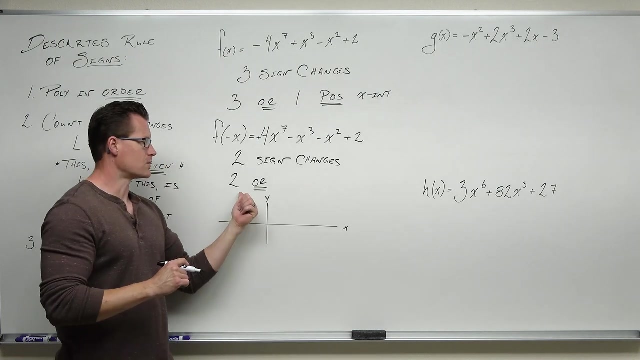 than that will represent your negative x intercepts. So here's what this says. This says: if I have two sign changes after evaluating negative x, I will have either two or start subtracting two and get your list down to either one or zero. I will have either two. 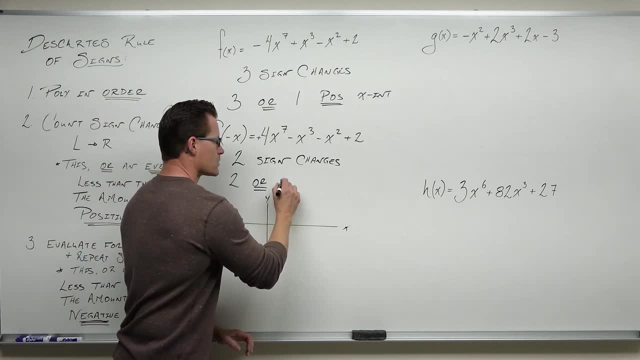 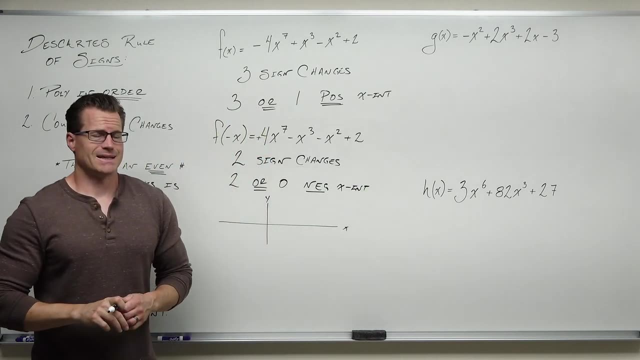 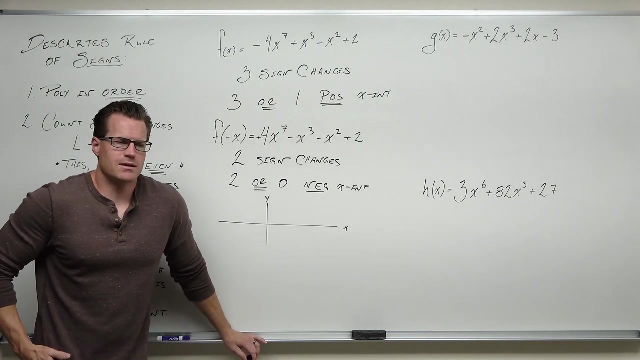 or zero. Two minus two is zero Two or zero negative x intercepts. That's it. That's all we can possibly have Now. why am I teaching this to you? Well, because if you use some critical thinking, this can really help you later. I want you to think about this: What's the degree of your 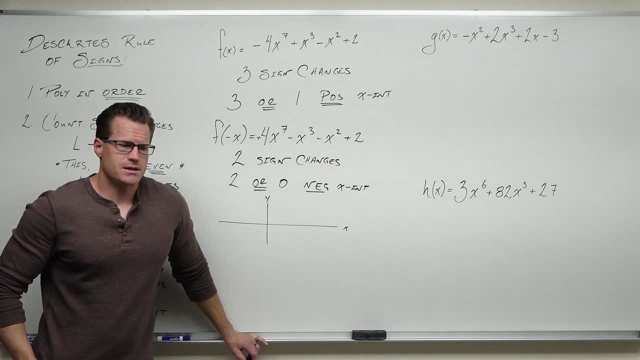 polynomial right now. You should look up there and go: that's seven. That says potentially the most we could have are seven x intercepts. That's it: Seven x intercepts. Are we going to have that many? No, and I guarantee it Here's. 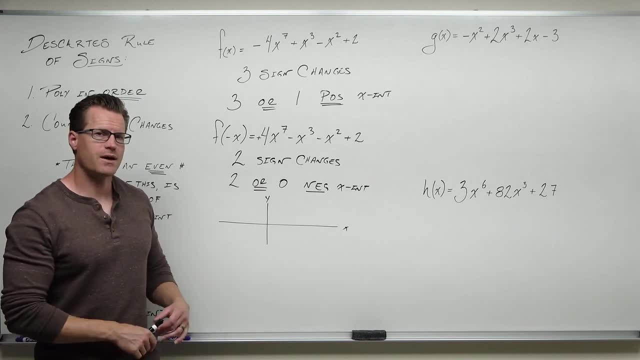 why We did Descartes' rule of sines and it says are positive x intercepts. There's either three of them or one of them. Notice how we subtracted two to get that list. We stopped at one because 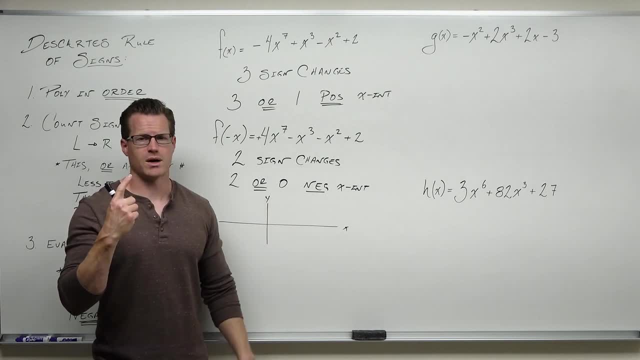 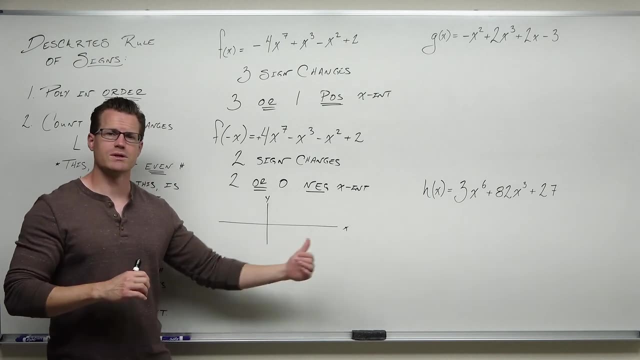 you can't subtract two past that. So we have either three or one positive x intercepts. We changed the sign over odd power terms and essentially evaluated negative x and we did it again. We said, okay, there's either two or zero negative x intercepts. You are either going to 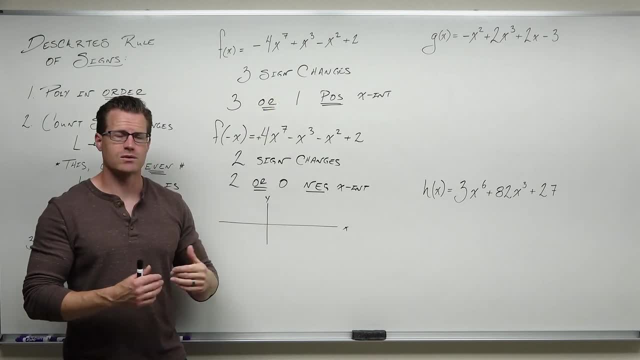 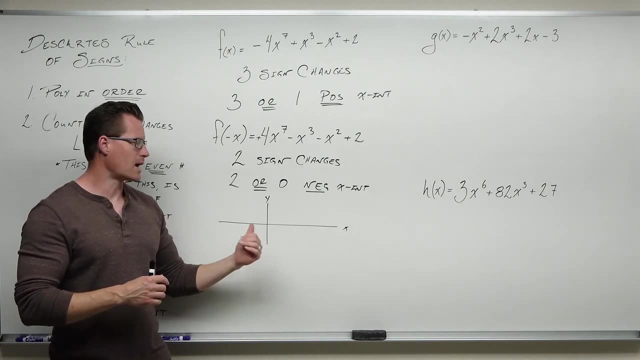 have positives or negatives. You can't think about it like that. You can't think about it like that. You can't factor out an x, and so there's no zero, There's no x. intercept right at zero. That's not going to work. So you either have three or one over here, two or zero over here. You could. 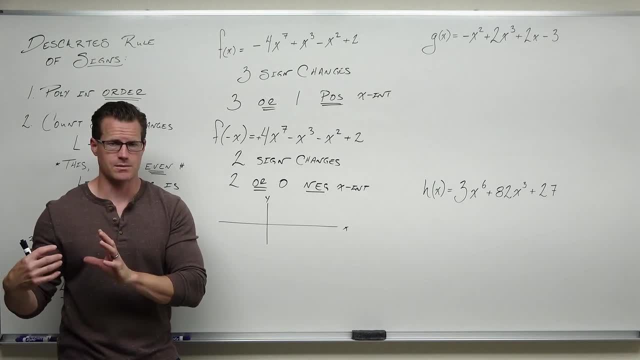 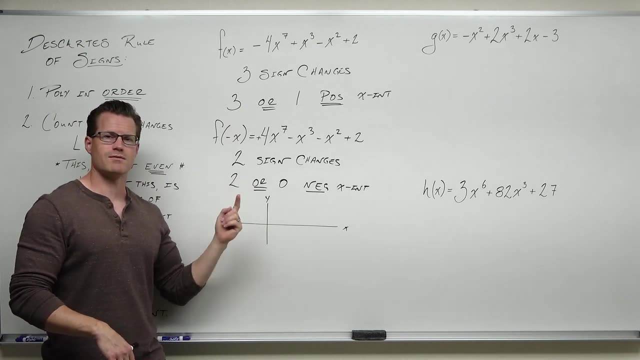 potentially have no x intercepts and negative x intercepts- none of them. but you definitely don't have seven. Look at this: At most you could have three positive and two negative. That's only five. That's only five. So if our degree is seven and we say we can have at most five, 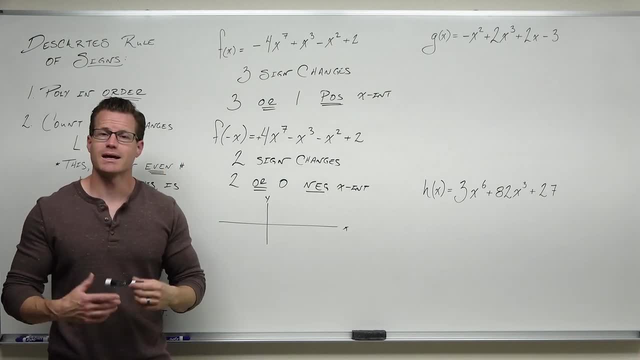 then what's the other two? The other two is something like x squared plus 25.. It will give you an irreducible quadratic that does not give you x intercepts. That's valuable to know. So we know that when we factor this, when we get down to factoring that one, we're going to end with at: 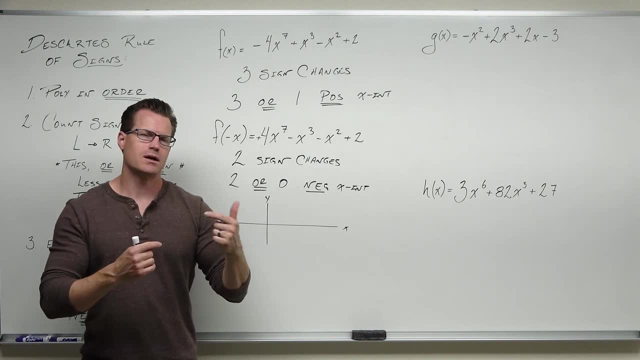 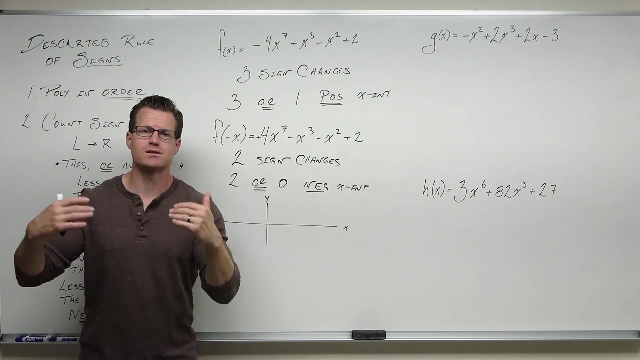 least one irreducible quadratic. Again, the irreducible quadratic because that is a power two that starts taking away two at a time from your degree. and the same thing would happen two at a time from your positive and or your negative x intercepts. That's why you subtract two to get 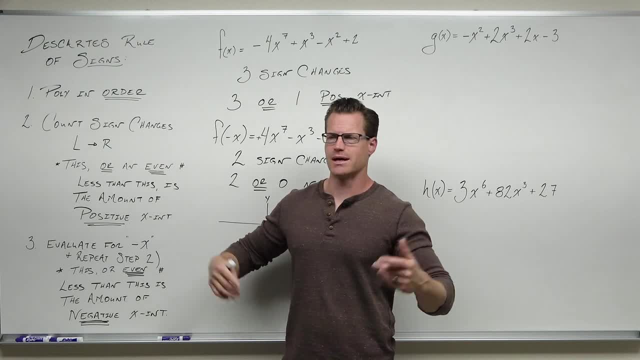 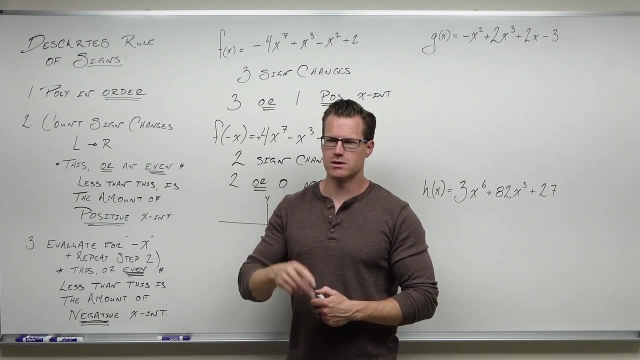 this list. It sounds really weird to say: subtract some even number less than that. Well, what they mean is: yeah, subtract two, then subtract two again. What do you subtract Four? Subtract two, then two, then two. What do you subtract Six? That's why it says an even number. It basically: 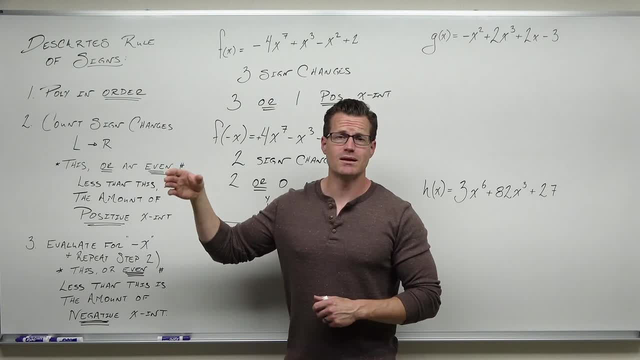 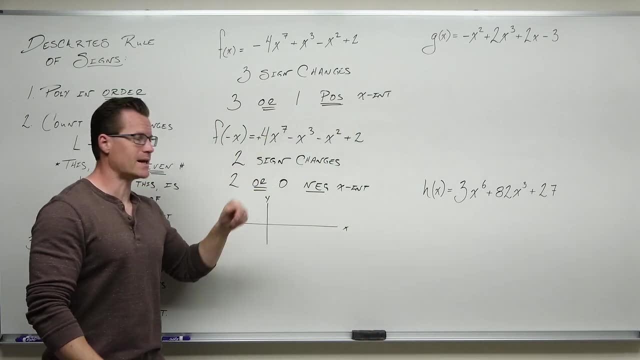 what it does. it says: just give me a list, Start with the number, sign changes. Give me a list by subtracting two until you get to one or zero, This or that, and then you're done. This is the potential of positive x intercepts. 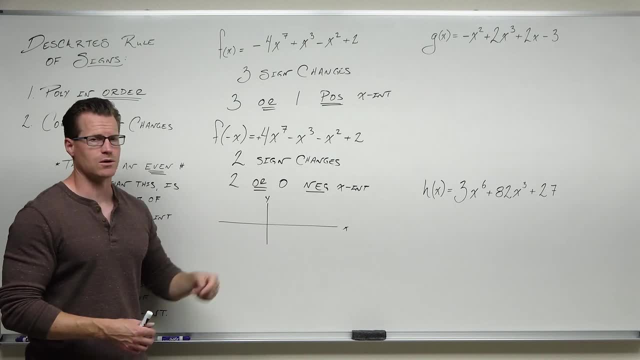 three or one, or potential of negative x intercepts, two or zero. It also says one more thing: If you find a negative x intercept, you know for sure that you have to have another one, because you're either zero or two. So if you find one of them, there's going to be another one. 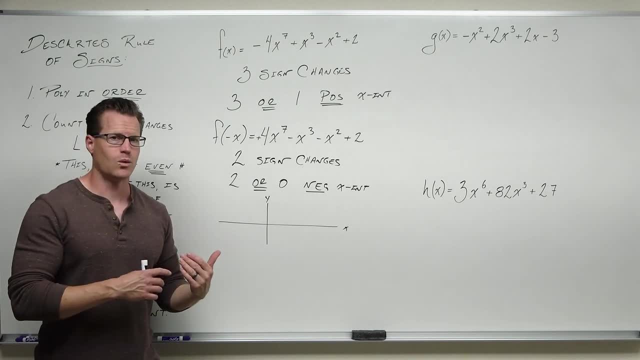 because you know you have to have zero or two. You can't find one and then go. I have zero. That doesn't make sense. You can't find one and go. I guess I have one. It was wrong. No, no, no. 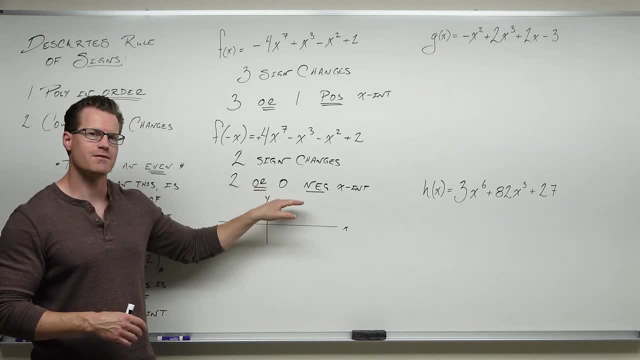 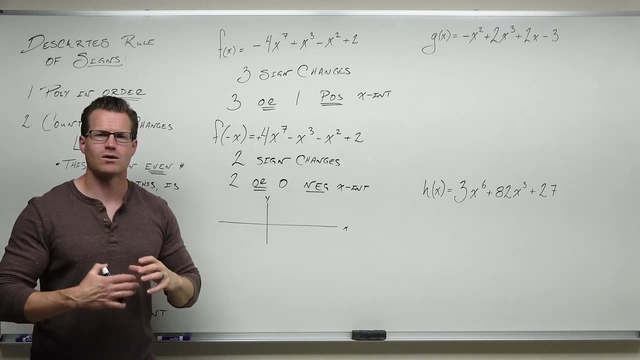 no, It's going to be either zero or two. So if you find one negative x intercept, there is going to be another one there, according to at least this polynomial. So that's the main idea. That's Descartes' Rule of Signs. As we move forward to the next section, I'm going to be refreshing your 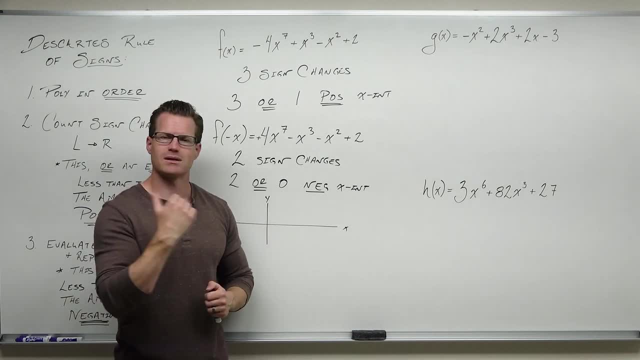 memory on this. We're going to do it every single time. So I'm going to say, hey, remember Descartes' Rule of Signs. Let's make this easier, Let's see what we could potentially have. I'm also going to 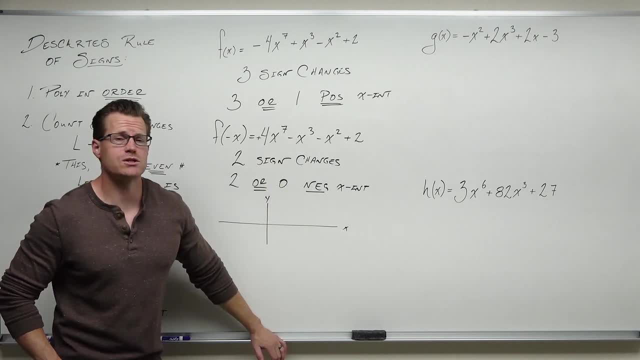 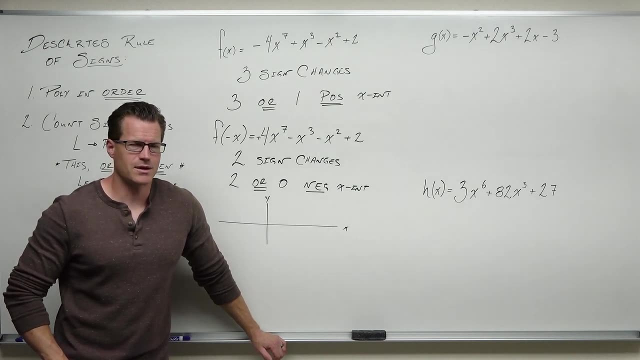 refresh your memory that in the last video that you watched we had those two examples and I hope you might pause and go back and just kind of think about what those were when we started checking with long division and synthetic division on what we got out of them. So I'm going to refresh. 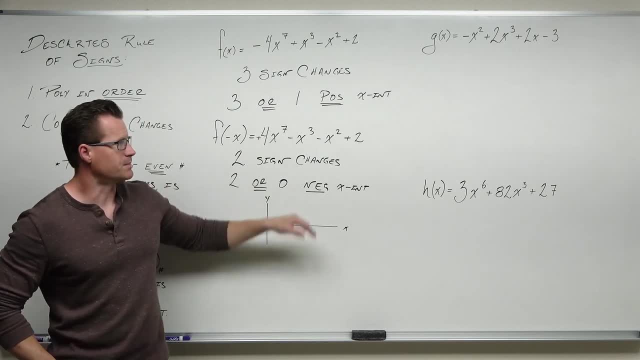 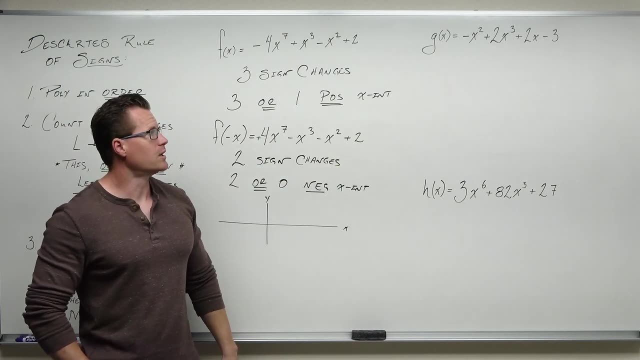 your memory as we go through. This is going to be interesting because it'll put this into play for you. So let's go ahead and let's practice Descartes' Rule of Signs two more times, just on these last two, and then we're going to call it good. So, G of x. hopefully you see what's wrong with this. 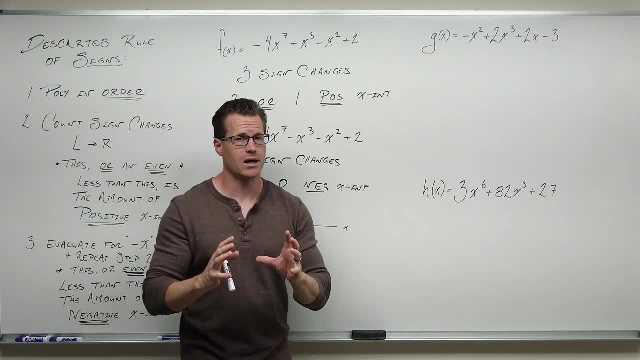 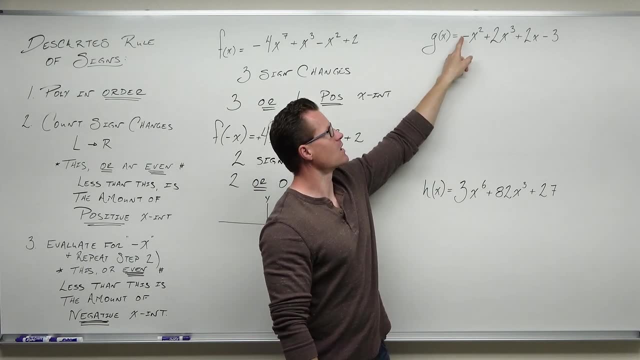 Before you start checking Descartes' Rule of Signs or anything that I tell you with polynomials, you have to have it in order. You see, if we go right from here and go, oh hey, yeah, this is a negative, that's a positive, that's one that doesn't change. 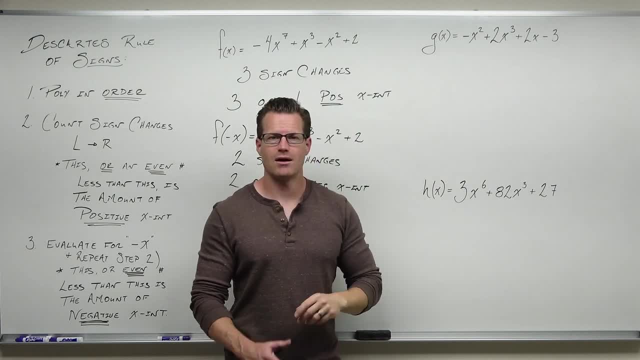 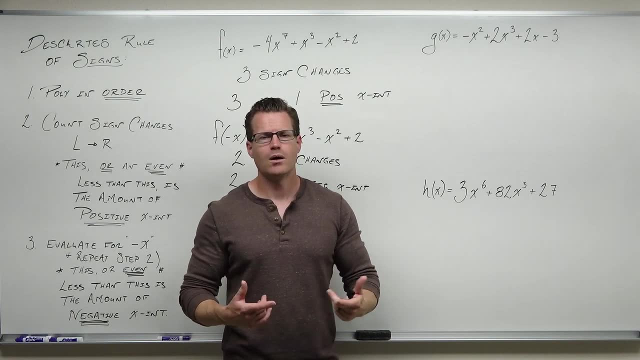 two sign changes. Hey, there's two sign changes. That means I would have remember I had not evaluated negative x. I would have two or zero positive x intercepts. That's wrong Why? Well, because this is not in order, and in order might change some signs around. And so when we put this: 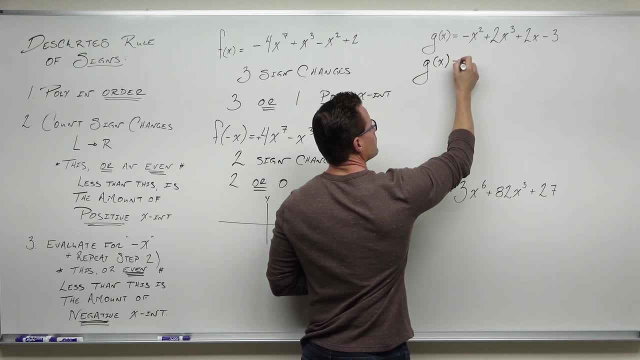 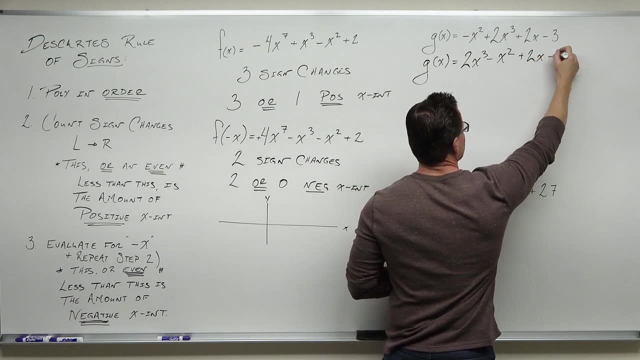 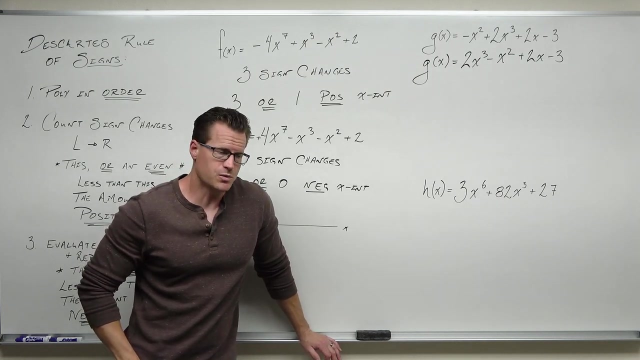 in order. when we put that in order, it is different. So let's think through everything I want you to know about polynomials at this point. Number one: they should be in order. Number two: well, when you look at the degree, that's like the first thing we look for is the leading term which has your degree. 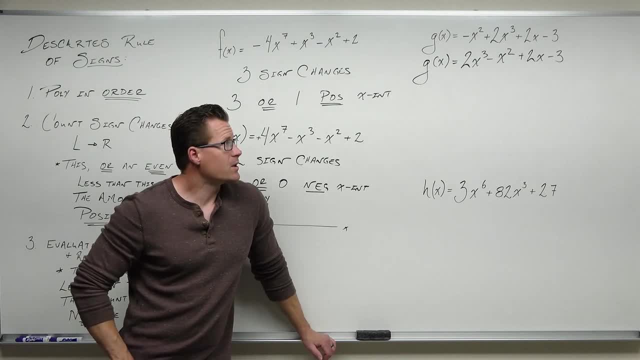 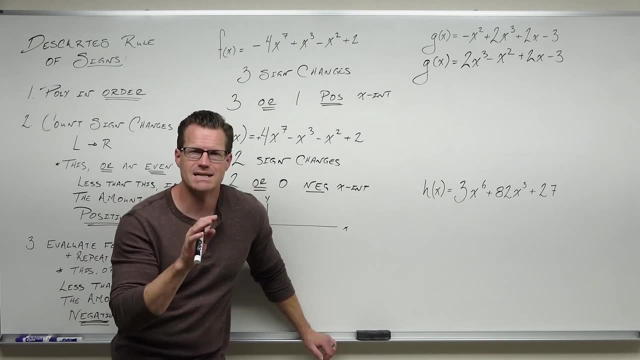 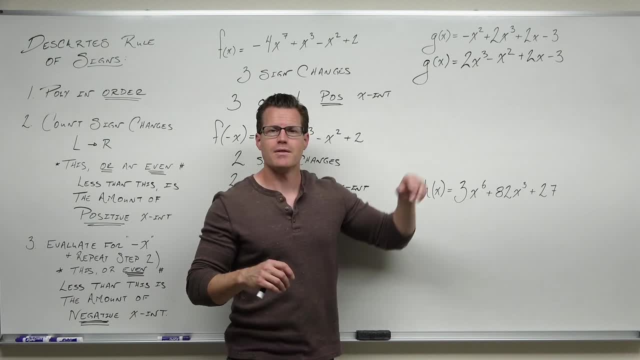 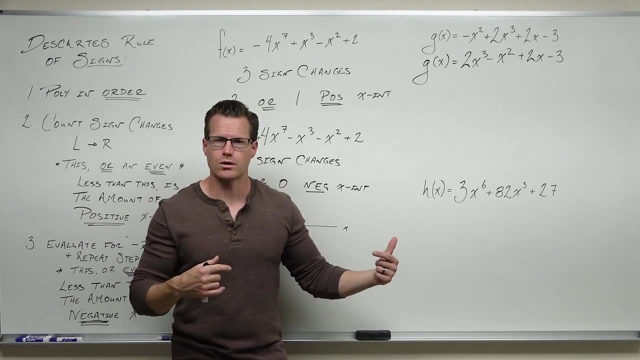 number of x-intercepts. So when I say, hey, three, this will have at most three x-intercepts, Is it going to have all three? You don't know without doing a little bit of work, and we're going to do. 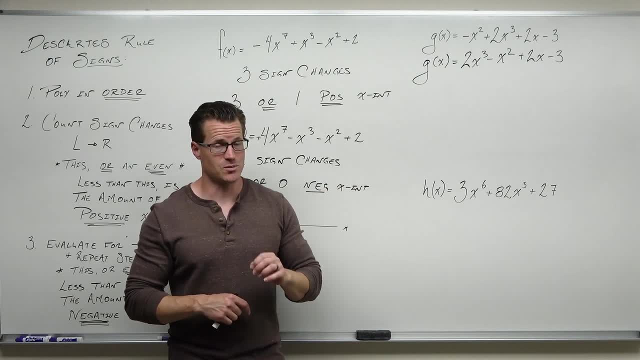 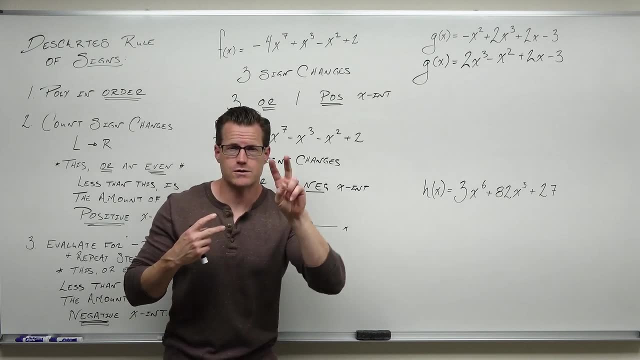 that work right now, But Descartes, Rules of Science will answer that question for us and it's pretty cool. So this will have at most three x-intercepts. What if it doesn't have three? Then pairs of two will be rounded out. So what if it doesn't have three? Then pairs of two will be rounded out. 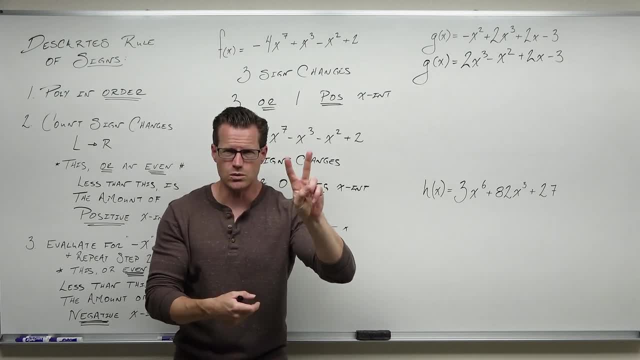 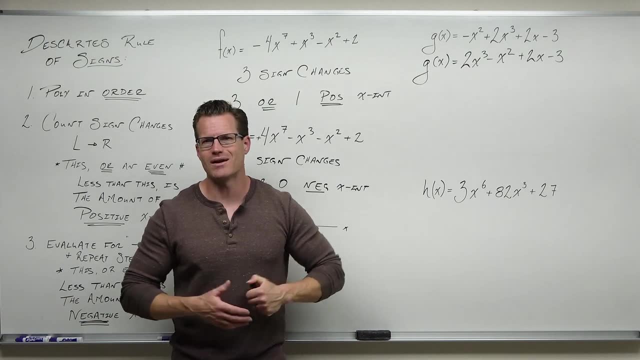 Packed up in irreducible quadratics, and pairs of two will be complex solutions. We're going to talk about exactly why that is. when we get two complex solutions, We'll say: why do they come in pairs, Why do they come in conjugate pairs? Has to do with quadratic formula and you get a plus. 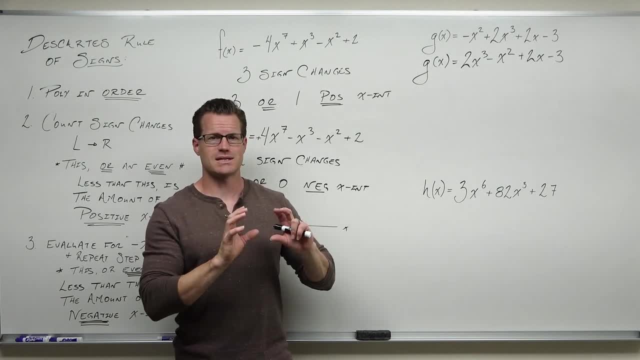 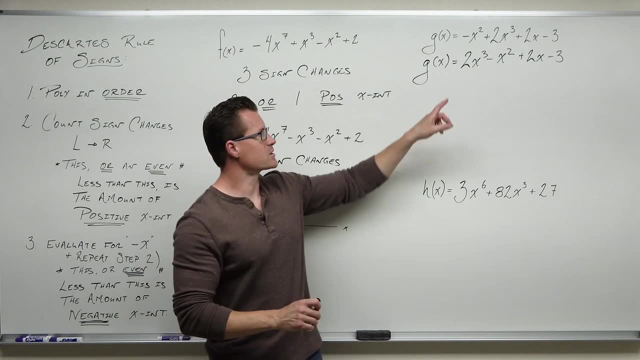 or minus and negative inside of a square root. Well then you get the same value, but plus and a minus You're going to get a conjugate pair. They always come in twos. I'm going to say that one more time. This degree tells you the maximum number of x-intercepts. 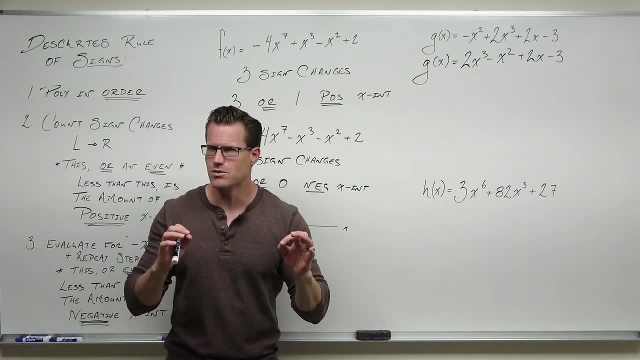 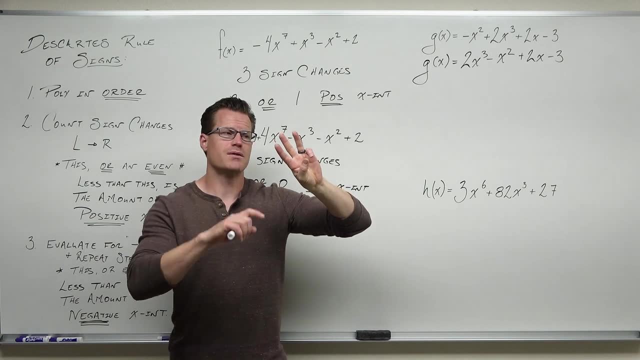 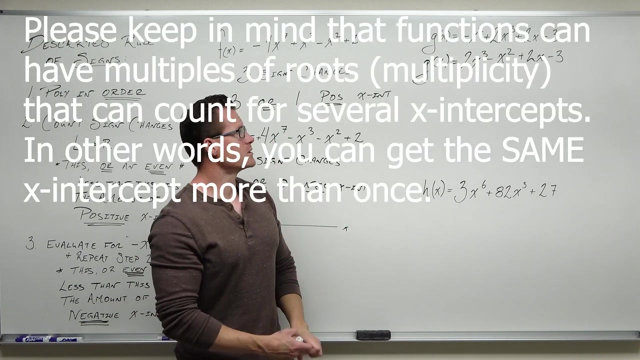 It tells you the total number of solutions if you have complex numbers. So we could potentially have three x-intercepts. If we don't have three x-intercepts, then we will have one x-intercept. They will be in pairs of twos if we don't have them. So let's go ahead and let's go through our. 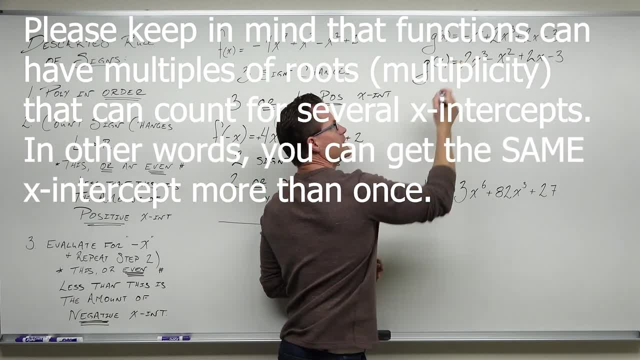 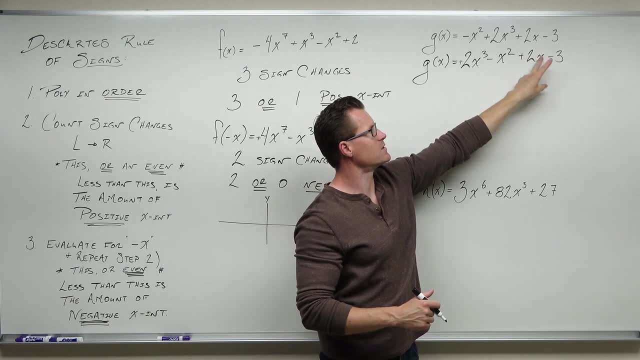 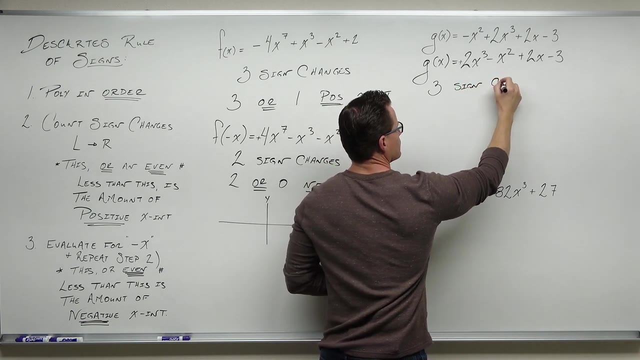 rules of science. So I'm going to put a little plus here so you can find that I start with a positive. Positive to negative, that's one sign change. Negative to positive: that's two sign changes. Positive to negative: that's three sign changes. What that means for us is that we are 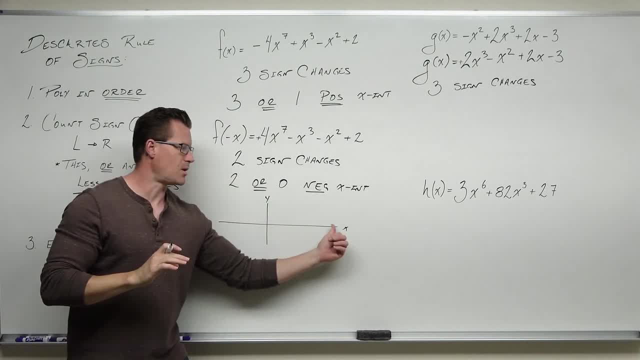 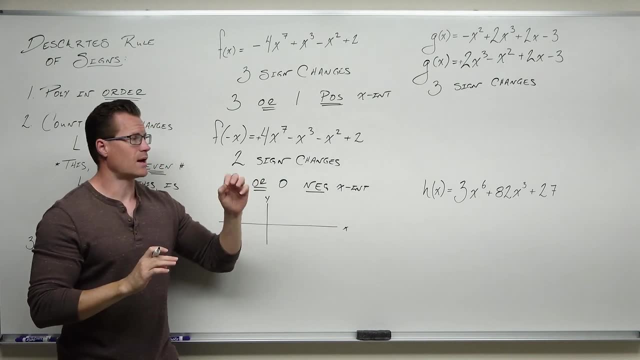 going to have three x-intercepts on the positive side of the x-axis, or subtract two from that number. create a list that goes down to one or zero. We'll have three positive x-intercepts or one positive x-intercepts, Nothing else. Those are the only x-intercepts that we're going to have. 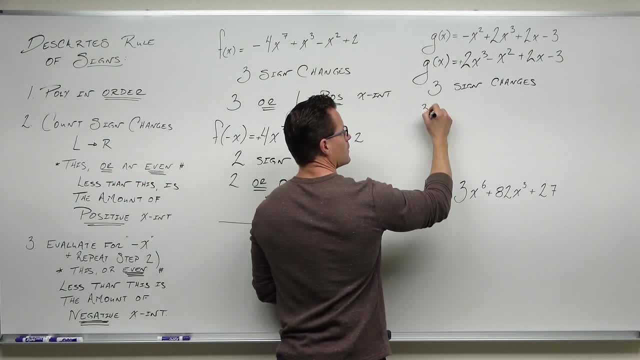 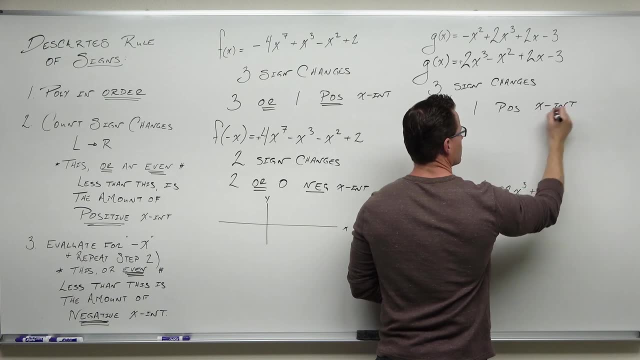 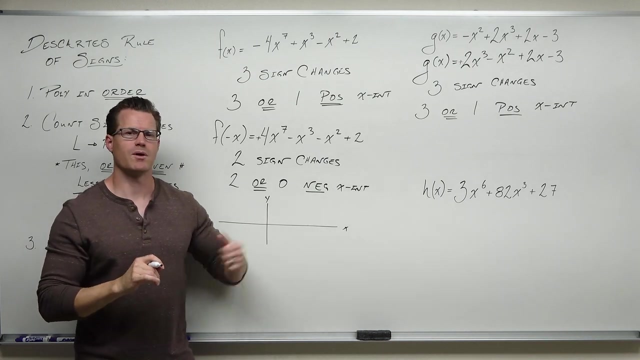 Only two options that you have here. So over here, we either hit it once or we hit it three times. No two, no zero. We know for sure that we're going to have a positive x-intercept, at least one, And so what we do in the next video. 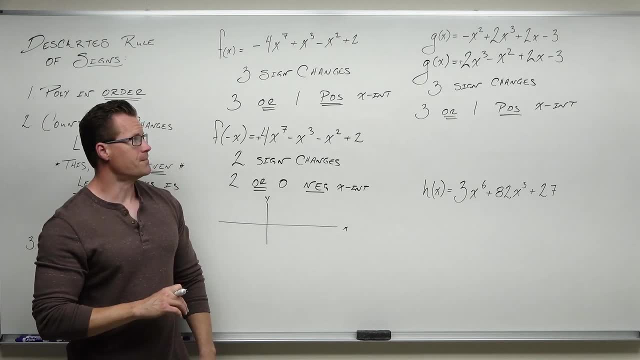 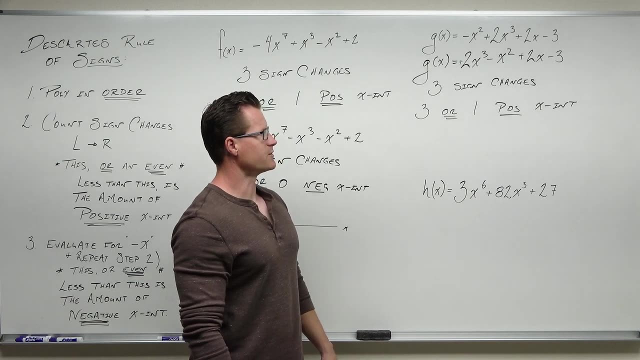 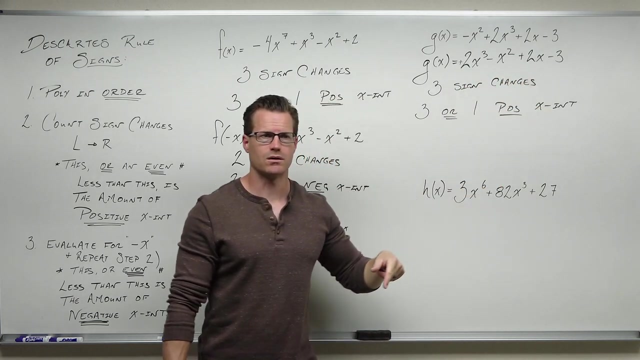 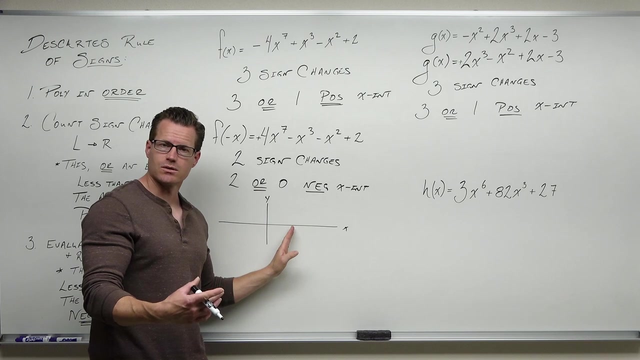 is, we would start checking positive numbers to see which one works. If you remember, we did that actually and we plugged in I think it was positive one. We said two minus one is one, One plus two is three, Three minus three is zero. Oh yeah, hey, one worked. One one is a positive x-intercept And we said that was a zero. 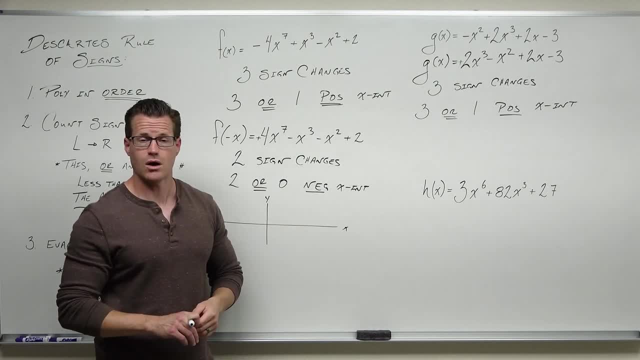 Therefore it gave us a factor and we did long division on that and I taught you synthetic division on that. So we knew we had one positive x-intercept. Now, what we got out of that- no, you know I won't ruin the suspense If you watch it back- what we got out of that was: 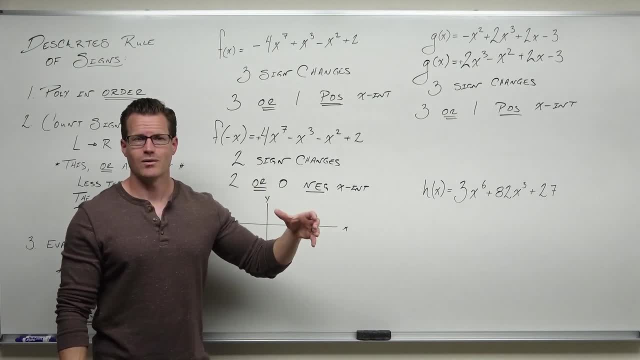 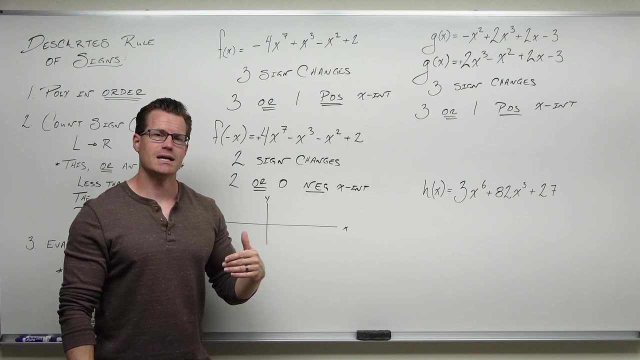 I'm not going to ruin the suspense. It was an irreducible quadratic when we got that. If you take that and you do synthetic division and just divide out one, use one as your x-intercept. what you're going to get is an irreducible quadratic. Wait a minute, do irreducible. 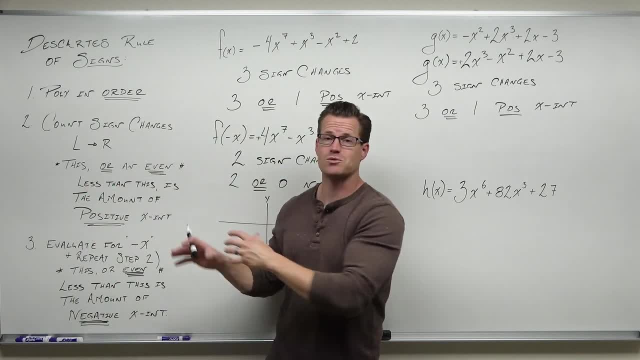 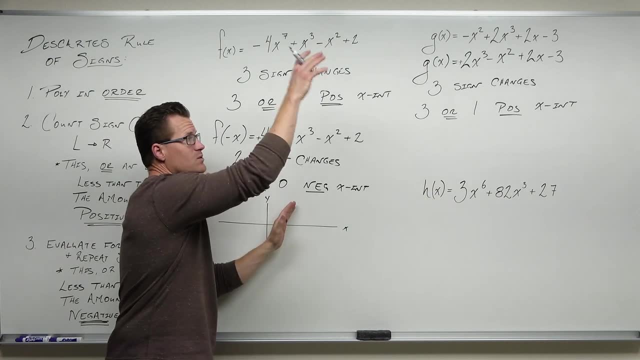 quadratics give you x-intercepts. No, that's the whole point of subtracting two. It was an irreducible quadratic. It gave you no more x-intercepts. So we found one positive x-intercept. What we did is we divided it and we found an irreducible quadratic that had no other x-intercepts. 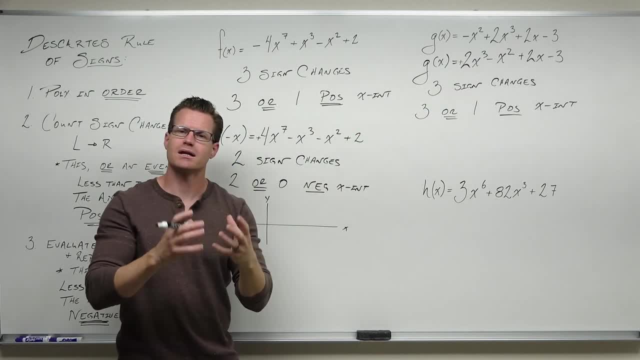 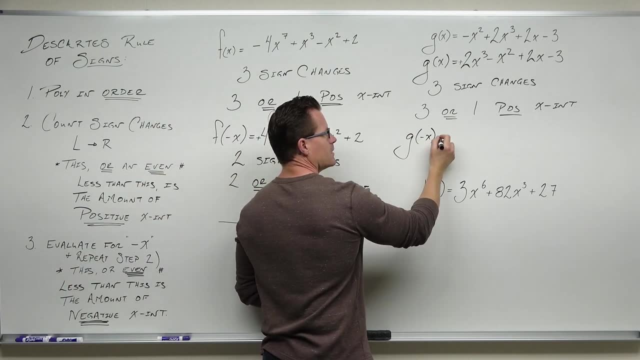 We can't have three here. Three is the maximum, but we got an irreducible quadratic. That was fascinating. Now let's go ahead and finish this thing off. If we had evaluated g of negative x, what we would do is we'd change our odd-powered terms, change the sign of those things. 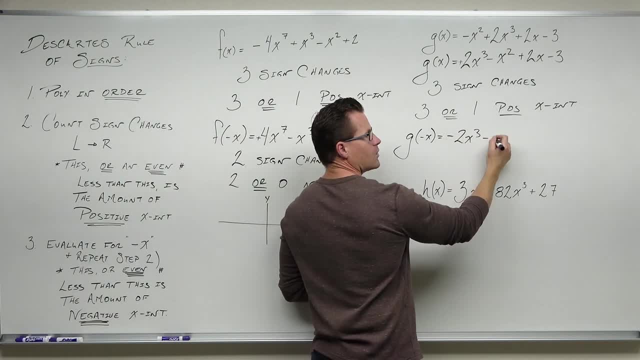 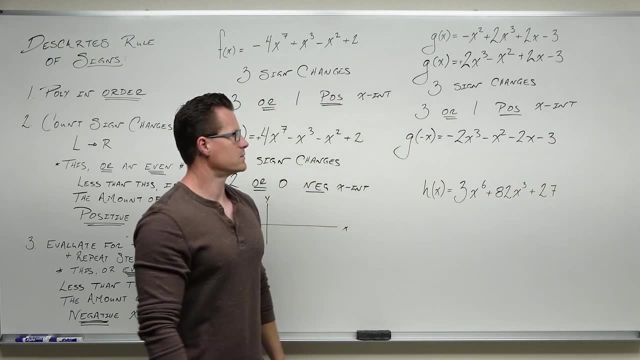 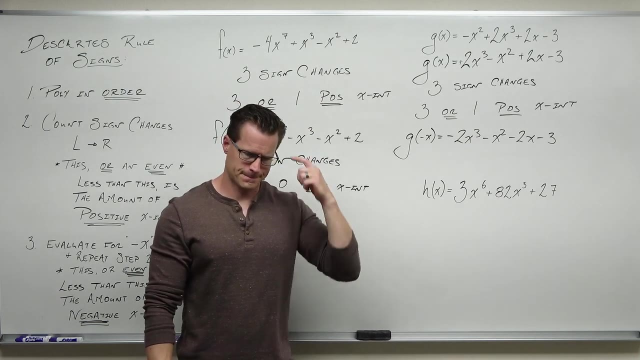 So we're going to have negative 2x cubed. We leave the x squared alone, Minus 2x. we leave the constant alone And you'll wait a second. hang on a second Negative, negative, negative. How many sign changes do you have? None, Zero sign changes. 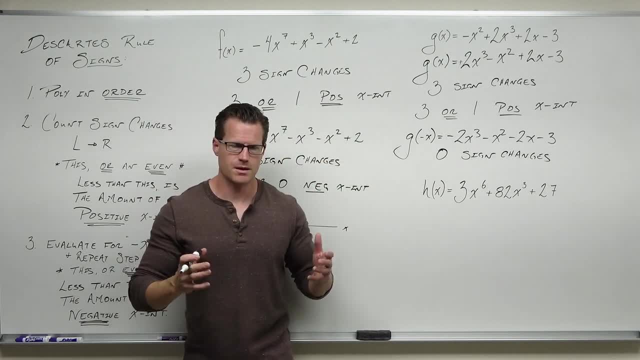 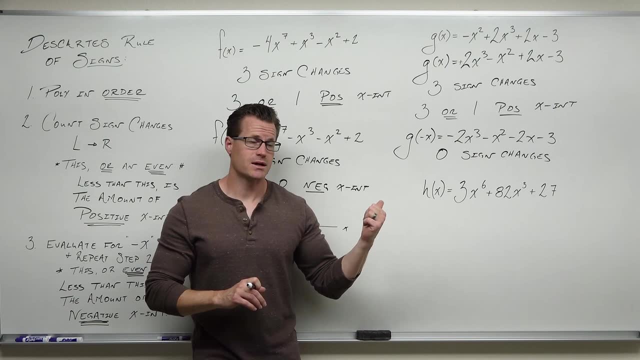 Now, this is where I think Descartes' Rule of Signs is very powerful. This is my opinion, This is where it's most powerful. If you have no sign changes, then that tells you something huge. That tells you in this case because, remember, we're on negative x here. This is talking about. 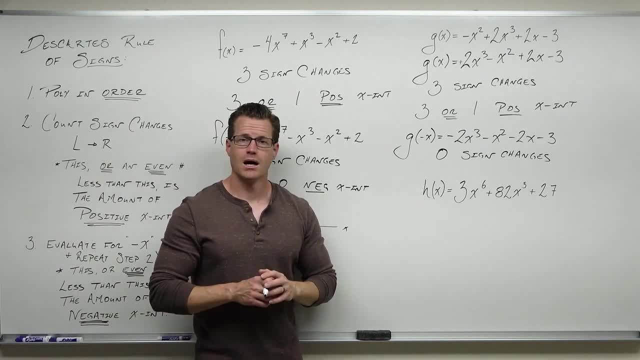 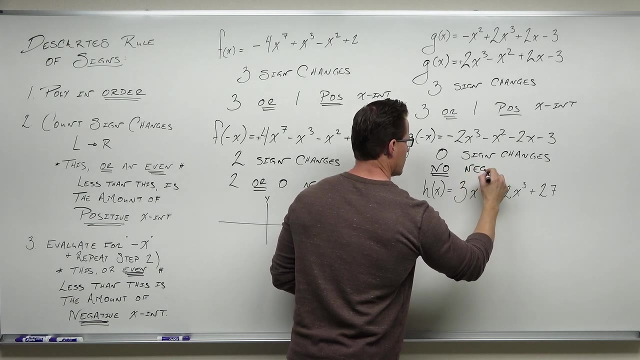 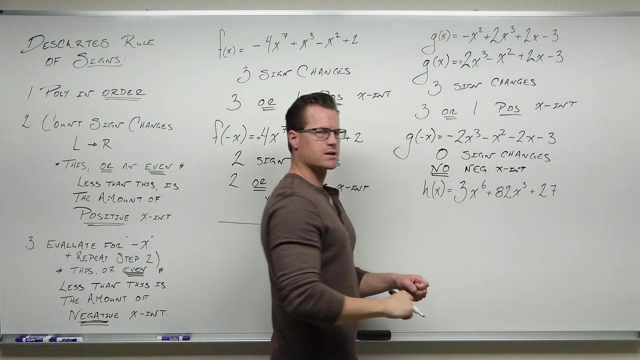 negative x-intercepts You are going to have how many? None, Not potentially two, not potentially four. None, You will have zero negative x-intercepts, 100% guaranteed. Now, if you're curious as to why that's so important, in the next video you're going to 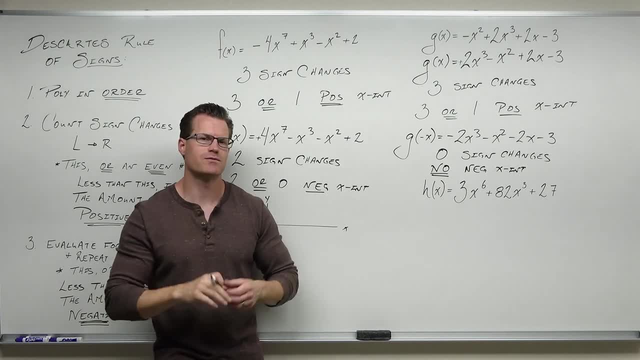 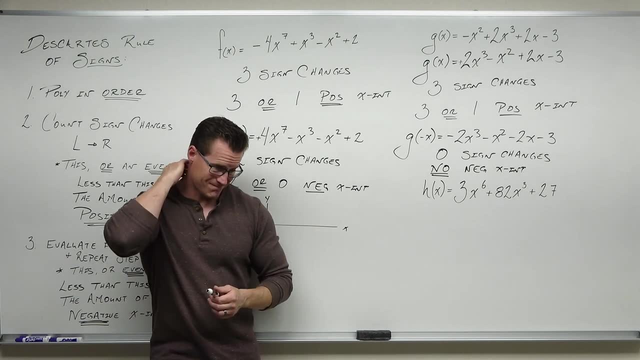 be learning something called the rational zero. You're going to be learning something called the numbers theorem, where I tell you how to find a list of numbers that are potentially or that contain all of your rational zeros. Well, if you know that you have no negative x-intercepts, 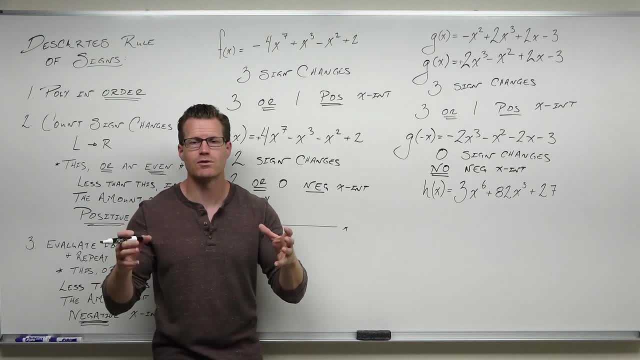 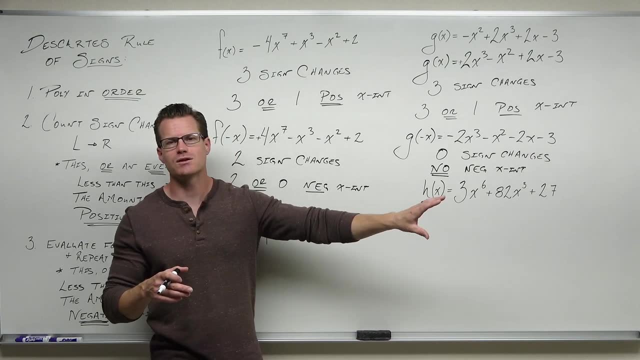 don't check negatives. That's huge. That saves you half of the work that you would otherwise do because you've got to check negative and positive. Normally, if you know you don't have negative x-intercepts, you eliminate half your list of numbers to check. That's fantastic. 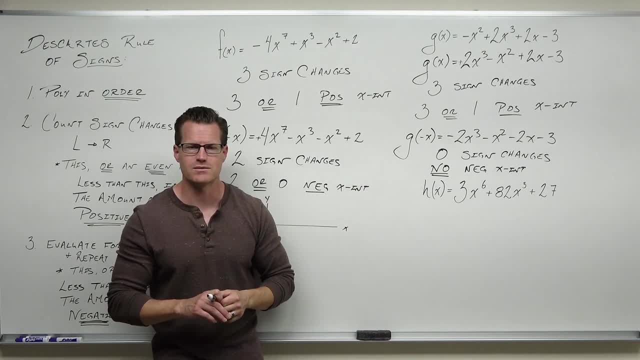 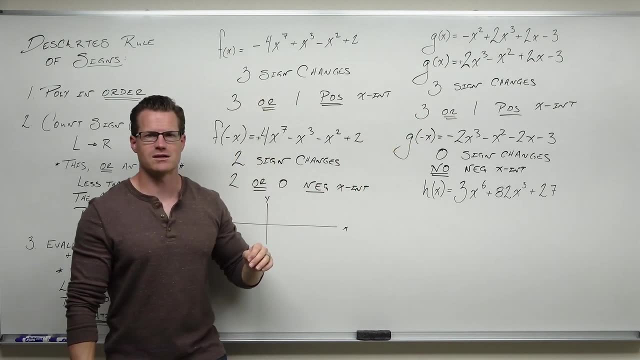 That saves you so much time because you're just going to be focused on the positive. so, wrapping this whole thing up with this example, we put it in order. We checked our sign changes. You say you have three or one positive x-intercepts. You change your odd. 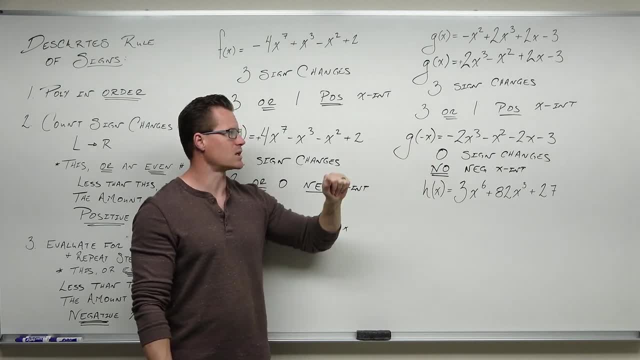 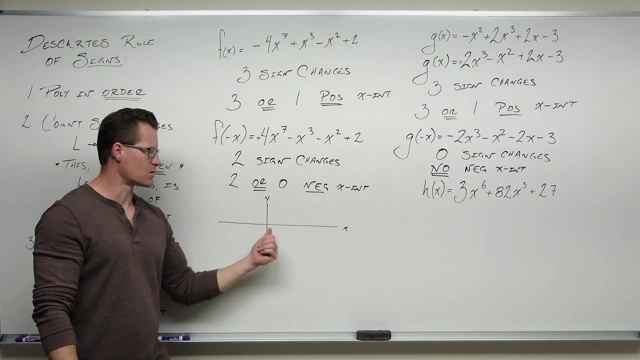 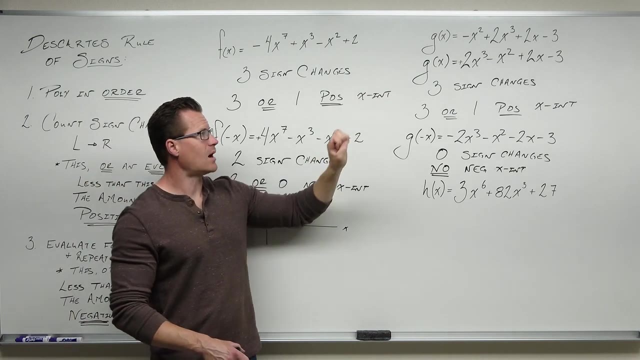 power terms by evaluating negative x and you have zero sign changes. This says you will have no negative x-intercepts. You either touch once or three times here. You are not going to cross over here. That's good to know. Then you start dividing Again when we divided out that one. 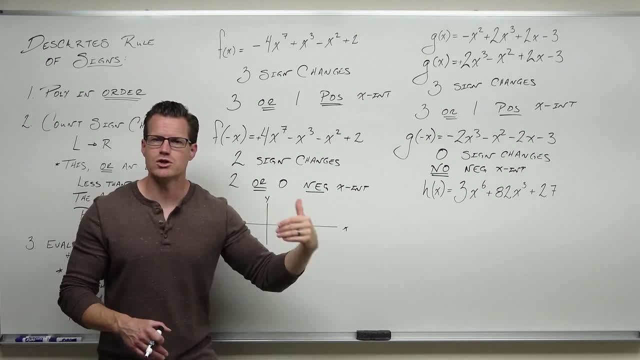 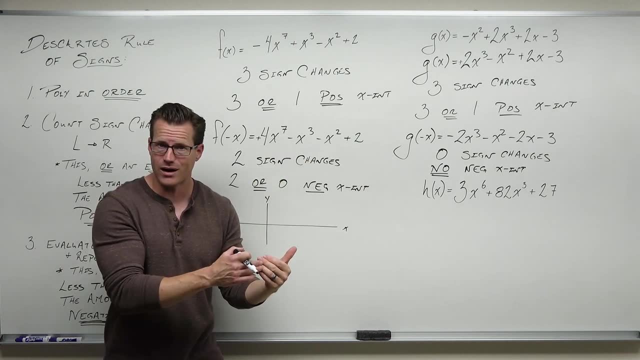 or that x minus one is the. we got an irreducible quadratic. What that means is that we are not going to have any more than one positive x-intercept. We found our one right. It was one. but when you divide that out and get an, 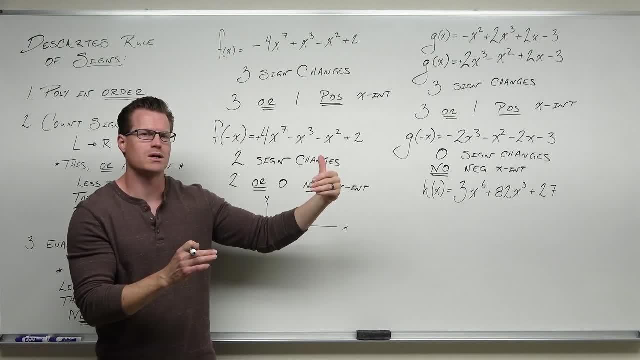 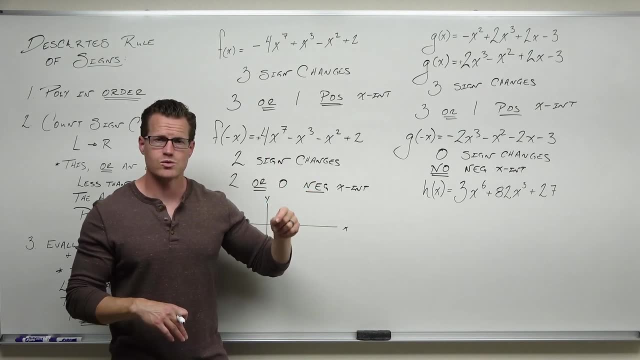 irreducible quadratic. it says, well, you can't go to three, You can't have two. That irreducible quadratic is why this happens, Why you go. you're either going to have three or one because that irreducible quadratic, while it took two away from your degree if you were to divide. 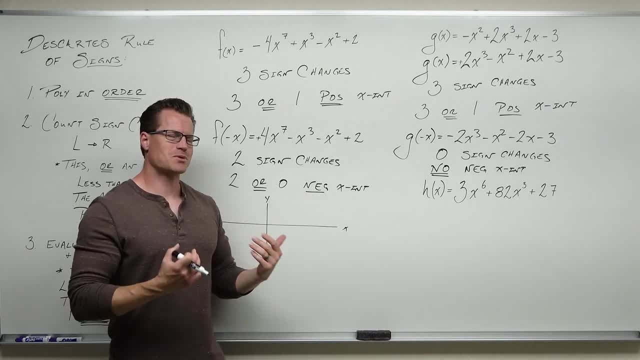 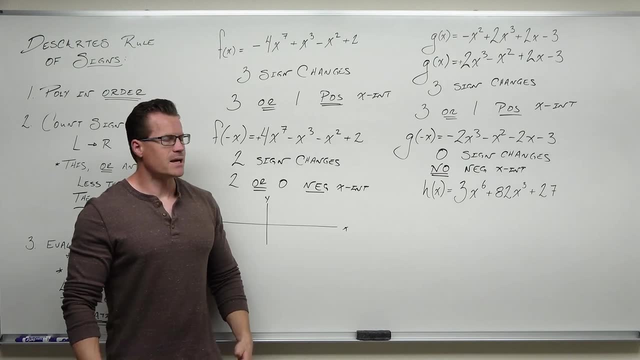 it. it doesn't yield any more x-intercepts. That's pretty interesting. I hope that that makes sense to you. It's very powerful and as we continue, you're going to see this thing play out. Right now it's just kind of an introduction on how it works and you're going 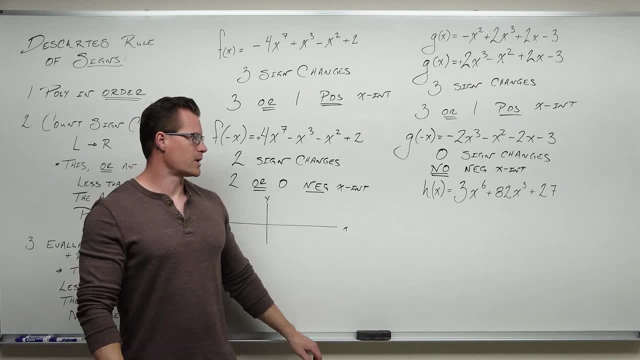 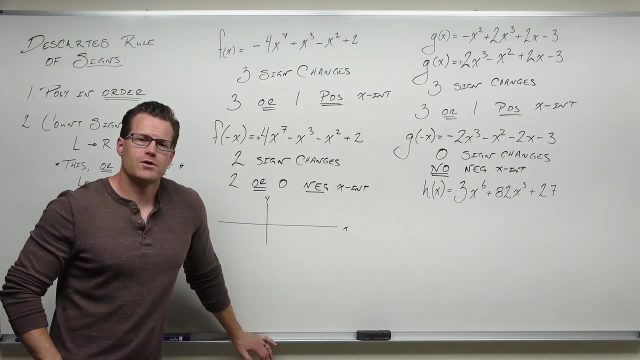 to see it in the next video. Let's do the last one. H of x is 3x to the sixth plus 82x to the third plus 27.. It's in order. That's really good. The first thing we do with the cart rule of signs. 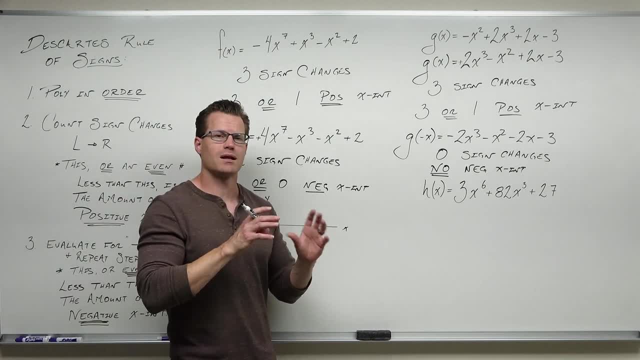 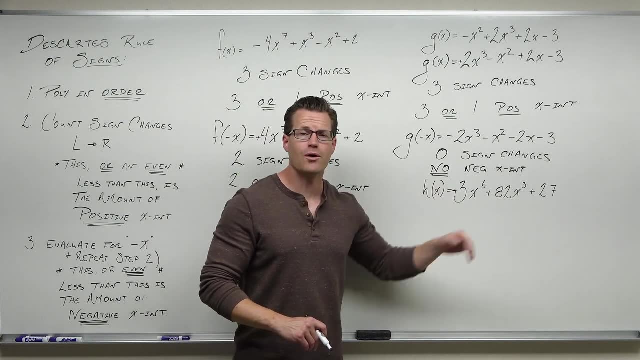 is. we count, the sign, changes the way that it is, and that will represent a list of positive x-intercepts. Wait a minute. That's a positive. That's a positive. That's a positive. There are no positive x-intercepts. What that means is that we have, or sorry. 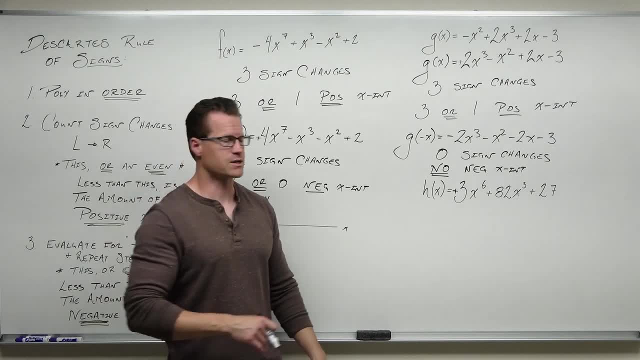 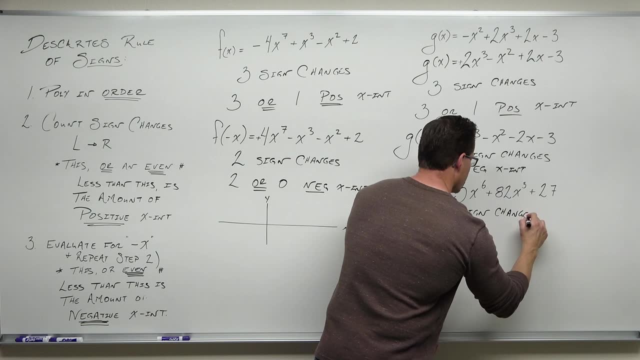 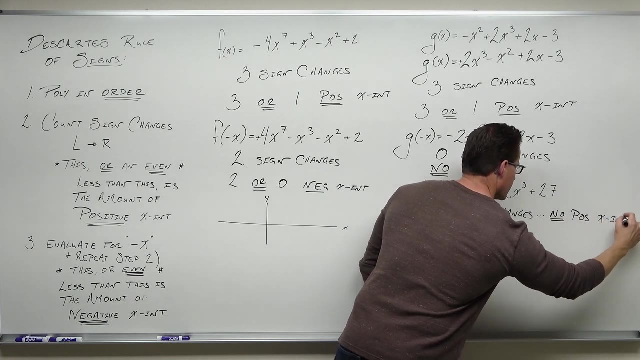 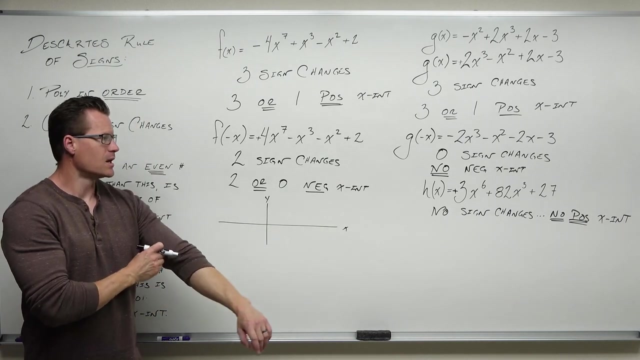 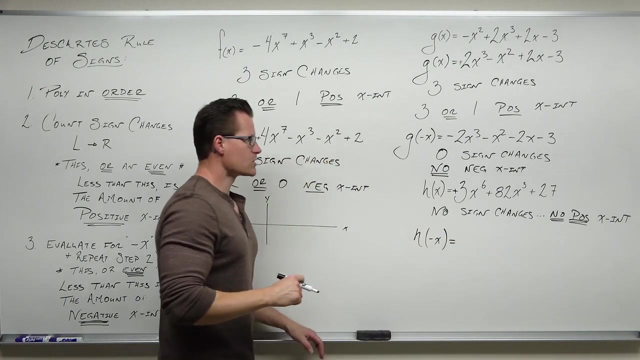 no sign changes. That means we have zero positive x-intercepts, None. This graph guaranteed will not intersect the positive half of the x-axis. Then what we do is we evaluate h of negative x. Essentially, that leaves your even power terms and your constant terms alone. It changes your 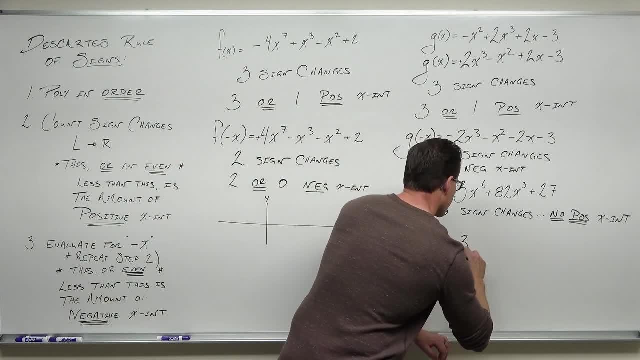 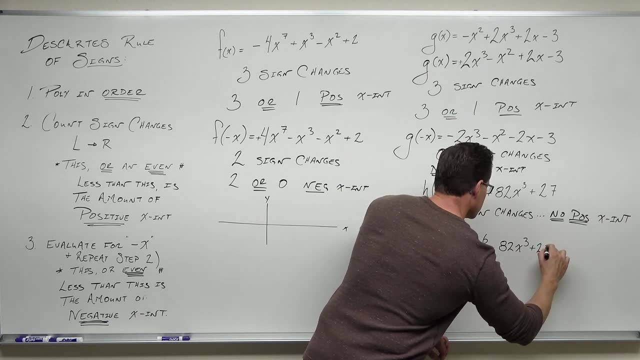 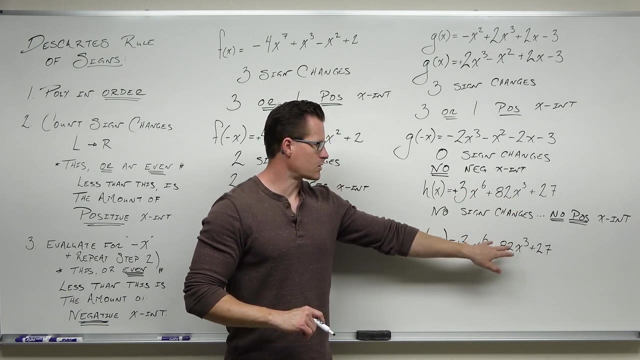 odd power terms due to the reasons we already talked about. So I keep my positive 3x to the sixth. That's an even power term. I change my 82x to the third. I change the sign because that's an odd power term. So even doesn't change, Odd does change. 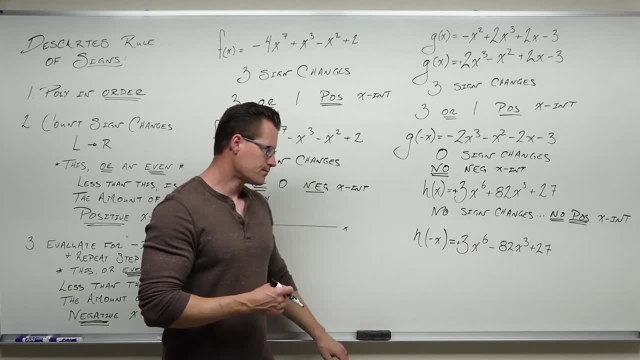 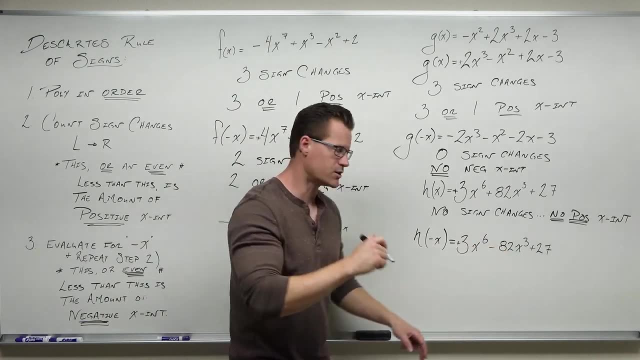 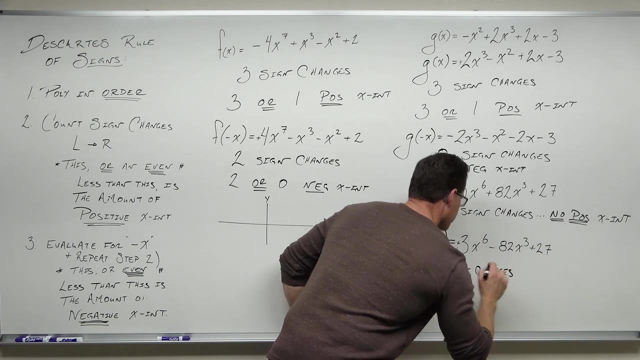 Constant was plus 27.. I leave it. Constants do not change. And so we now check our sign changes again. Positive to negative, that's one sign change. Negative to positive, that's two sign changes. Now what's it mean? I hope you were listening to the whole video. I gave you a lot of explanation. 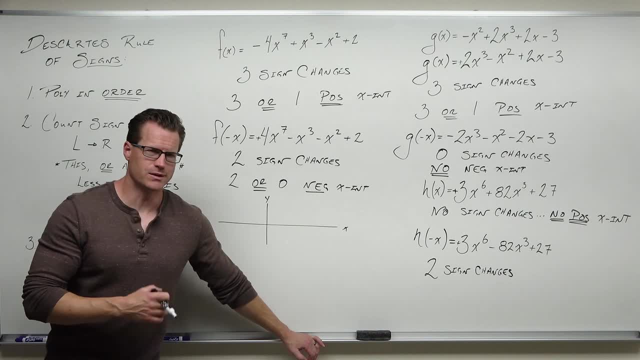 about why this stuff works how it works. I don't want you to be like, oh, I don't know, I don't know. I just want you to be able to do it. I want you to understand it. I want you to understand the. 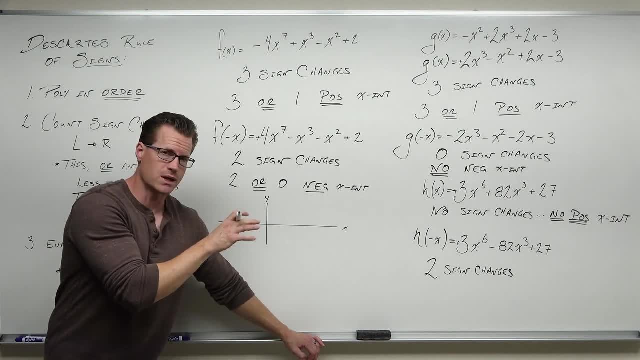 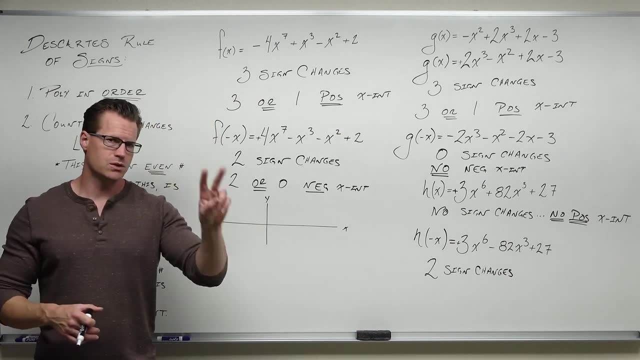 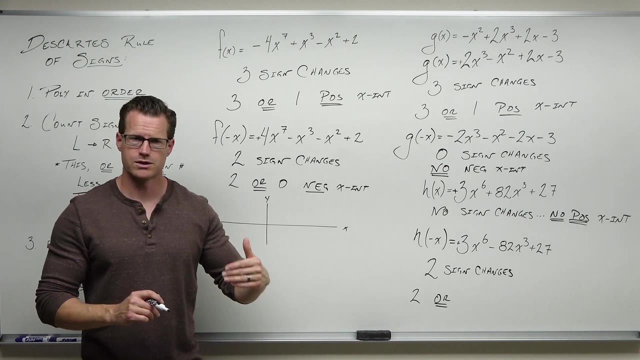 interplay between irreducible quadratics, the degree and why we subtract 2.. I want you to get that. So two sign changes means we will have either 2 or subtract 2 from that number until you get down to 1 or 0. So 2 minus 2 is 0.. 2 or 0. negative x-intercepts. 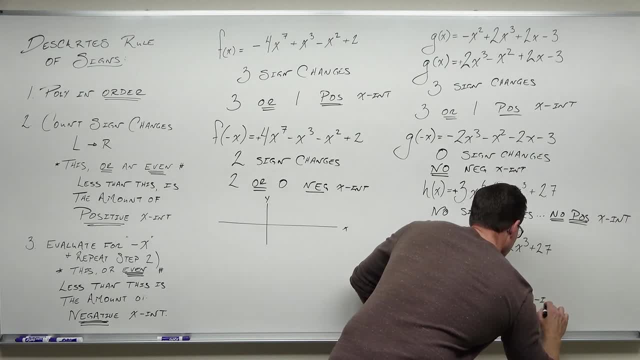 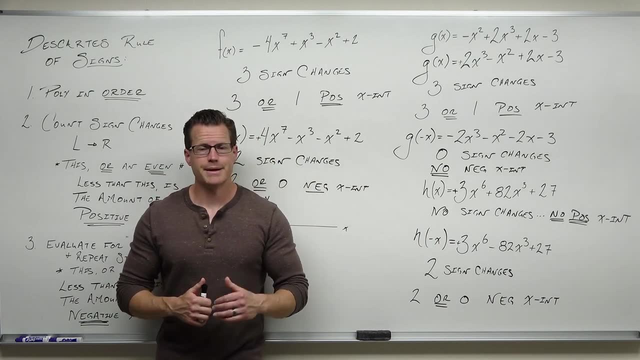 Now, if you remember, back to the previous video, we evaluated negative 3.. Negative 3 was an x-intercept. Remember that. Negative 3.. If you don't, maybe go back and look at your notes, look at the last. 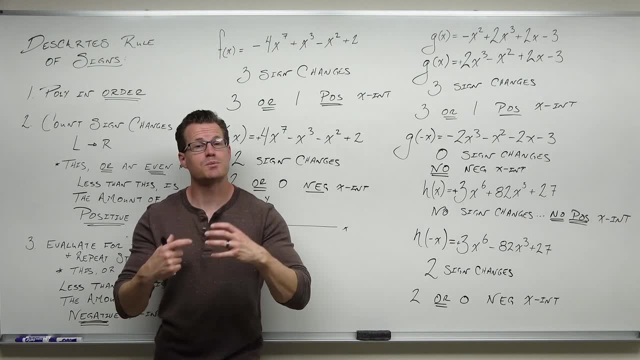 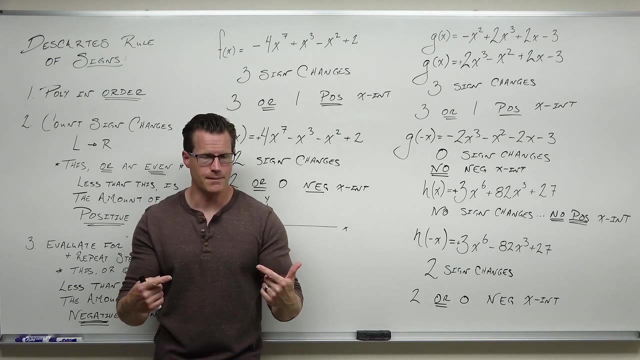 video: Negative 3 worked. We factored out x plus 3.. Remember, negative 3 would give us x plus 3 as a factor or synthetic division. We used that negative 3.. And we got another negative 3. It was a power 5. It was a degree 5 polynomial that we got out of that. We know for sure that. 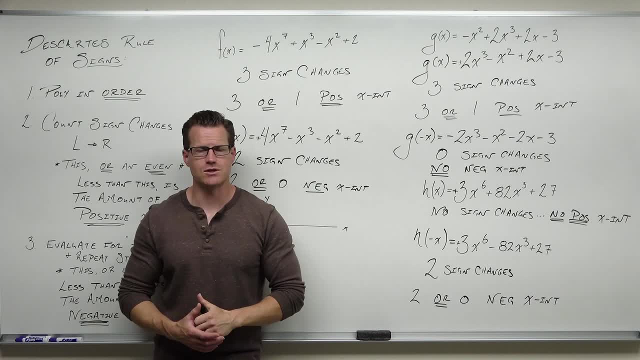 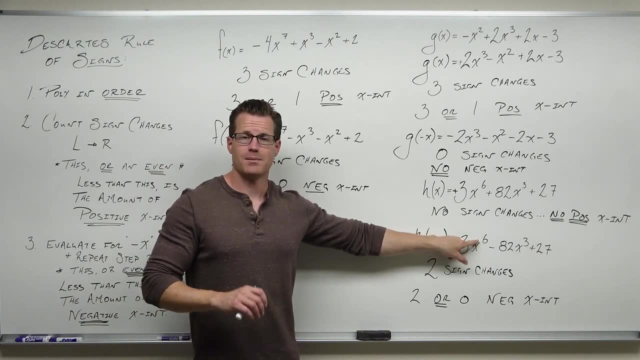 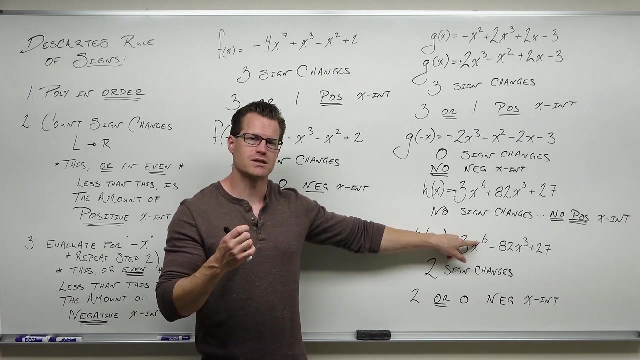 odd polynomials have to cross, don't they? They have to somewhere, at least once. So let's wrap this whole thing up. This last thing I'm going to talk about, that's a degree 6. It potentially has 6 x-intercepts. That's the most it could have. Does it have 6 of them? Well, no, This has 0. 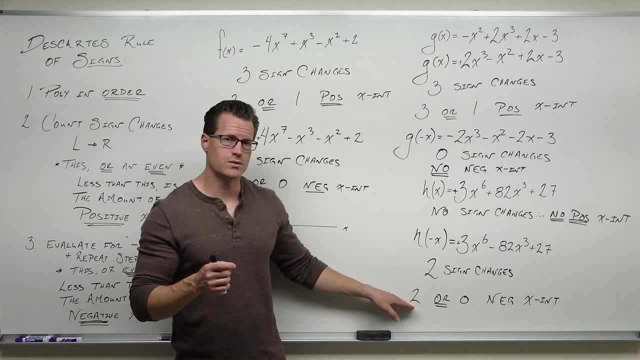 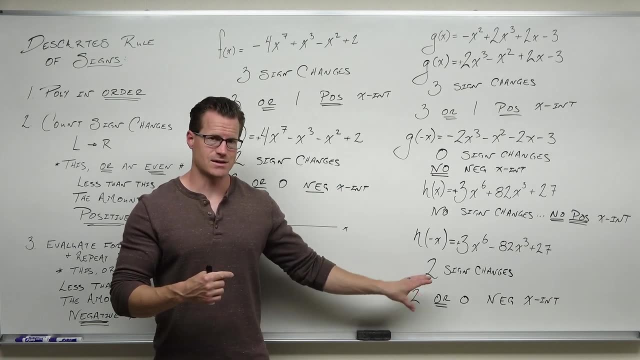 positive. This has 2 or 0 negative, So the most it could have is 2.. Now what did we learn in the last video? We learned that negative 3 is an x-intercept here, So wait a second, We found an x-intercept. 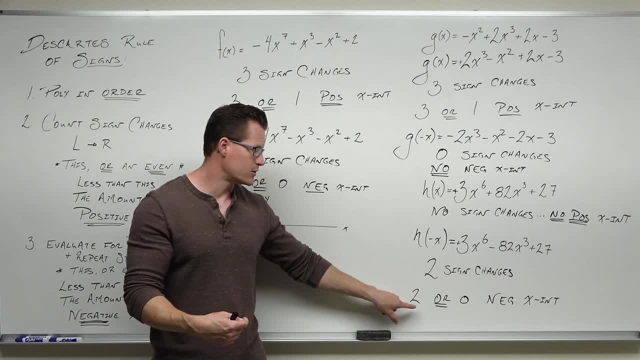 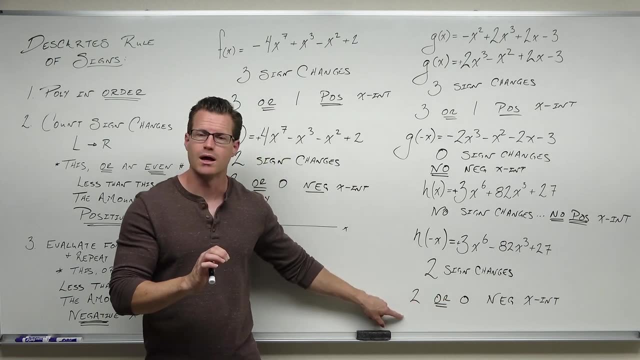 that was negative, So it's not 0. Therefore, it has to have 2.. Exactly, 2.. Did you get that? If we found 1 negative 3, then it can't be that one, It's got to be this one. There will have to. 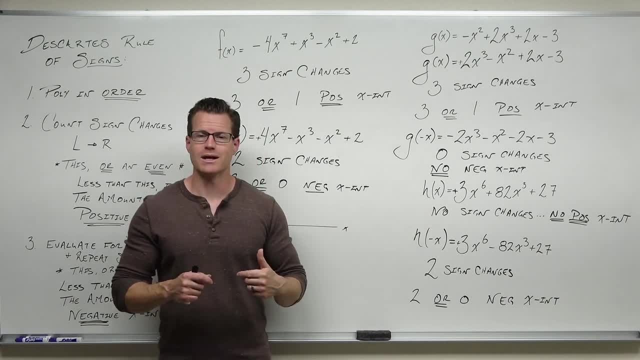 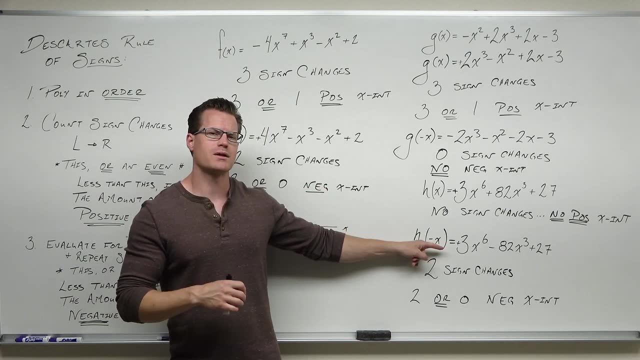 be another x-intercept on this besides the negative 3.. And we kind of sort of knew that because we ended with a degree 5 polynomial. If you factor out x plus 3 from here- maybe try this on your own synthetic division or something- then you're going to get. 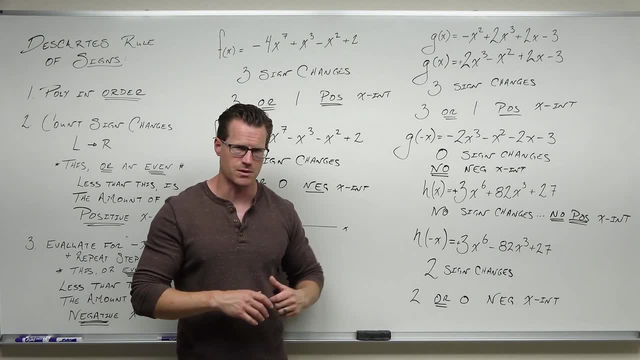 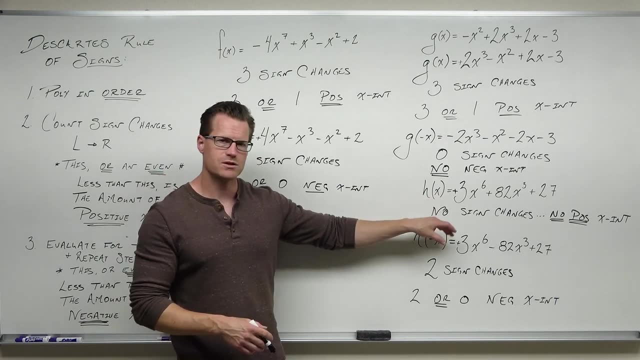 an x to the 5th, 3 x to the 5th, something, something, something, something. Well, that is still odd. That means it would have another x-intercept, And so that bears this out. No positives: We found 1 negative x-intercept, negative 3. We know there's another. The degree 5 says that. 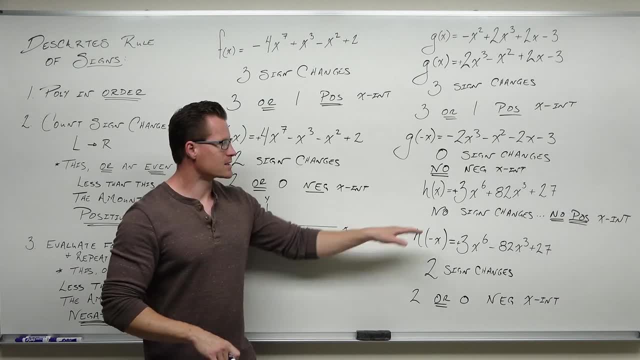 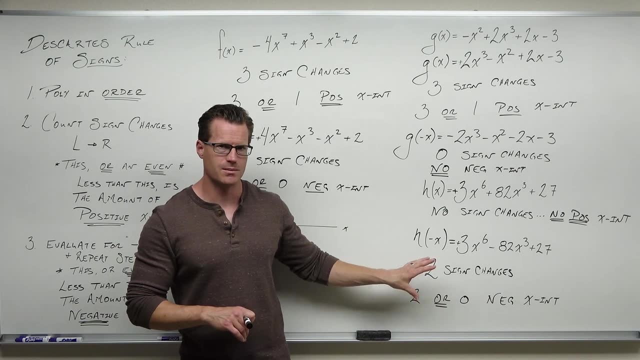 But after we find it we're going to be done. Why? Because there's no positives And there was at most 2 negatives. Maybe listen to that last explanation of this a couple times and tell the interplay between degree: most number of x-intercepts: 0 positives. 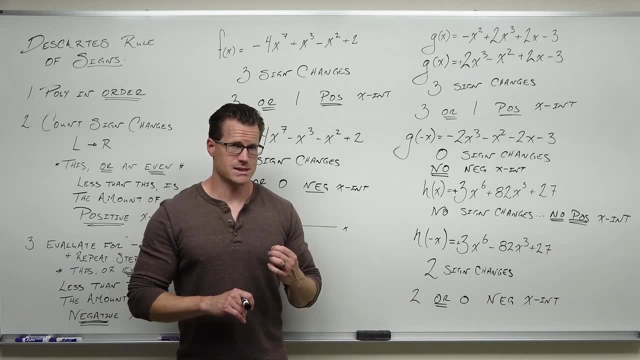 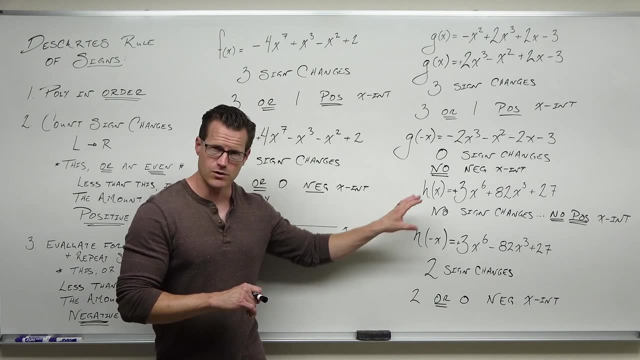 and 0 or 2 negatives And what we found makes sense. We found negative 3. That's a negative x-intercept. That means you can't have 0. You have to have 2.. We also, if you divide it out, 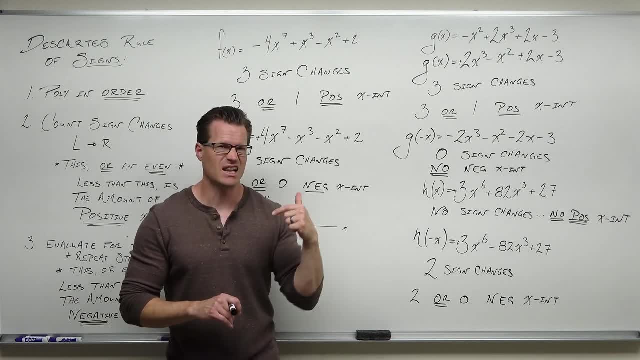 we get x to the 5th power. What that means is that we would have at least one more x-intercept, Because that's an odd, It has to cross, And then that would say, yeah, that's 0 to 1.. But 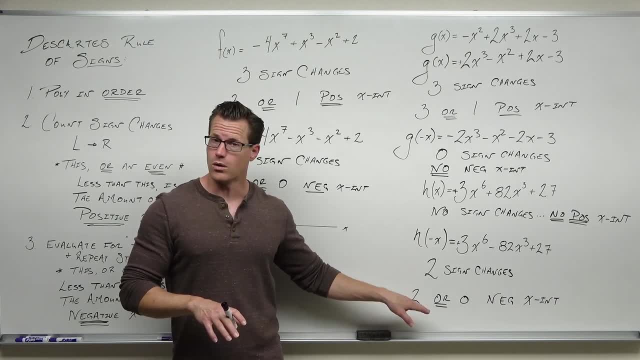 after that you're done, There's no 0s and there are no more negatives than the 2 that you would find. That's how the decartical assign is going to work for us. We're going to use this a lot. 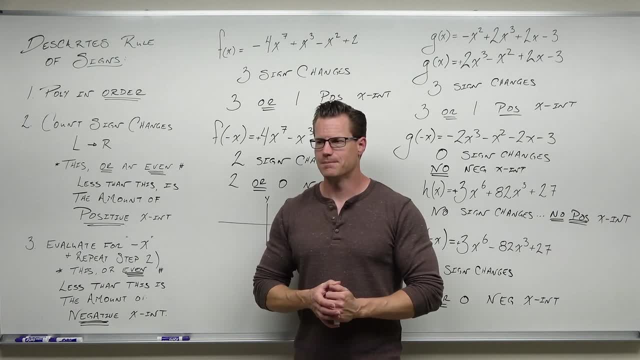 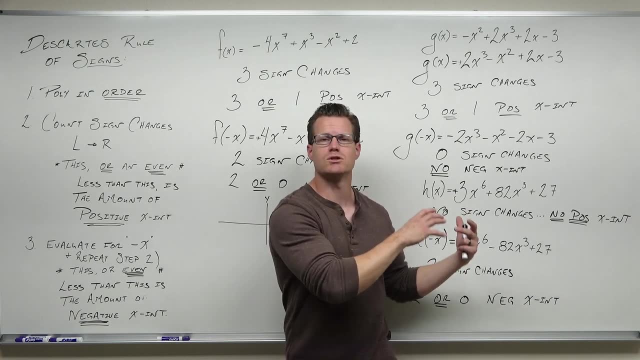 as we go forward into the next video, Every example that I do, I'm going to reference this, So you're going to start seeing it as we work it out, As we actually do: the long division or synthetic division. So I hope it makes sense. Maybe watch the last explanation of a couple. 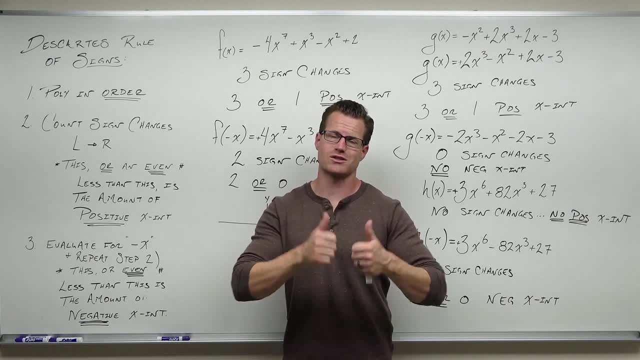 times until you really get that to click, If it hasn't already, if it has, awesome, And I will see you for the next video.